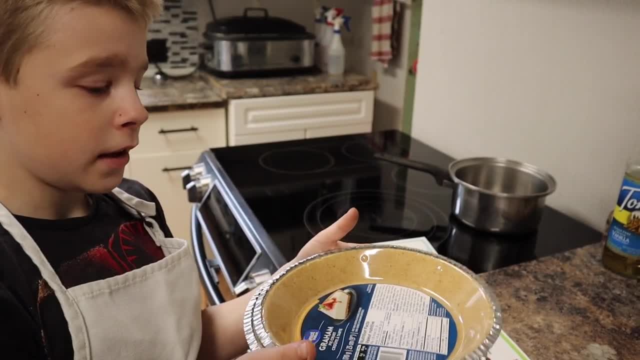 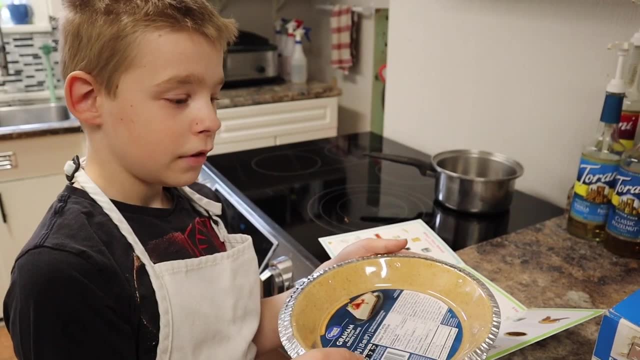 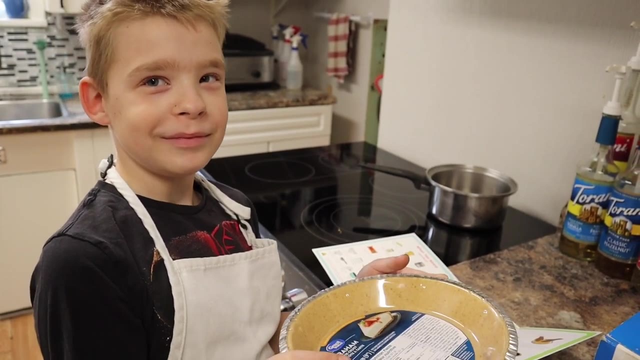 tonight. Yep, Okay, and, and these. if you cut it like this, it'll only fit four. Well, I was going to eat a whole pie, and then you- the rest of you- are going to share the other one. No, I want to eat a whole pie too. Oh, so you and I are the only ones having dessert, And the other kids with the. 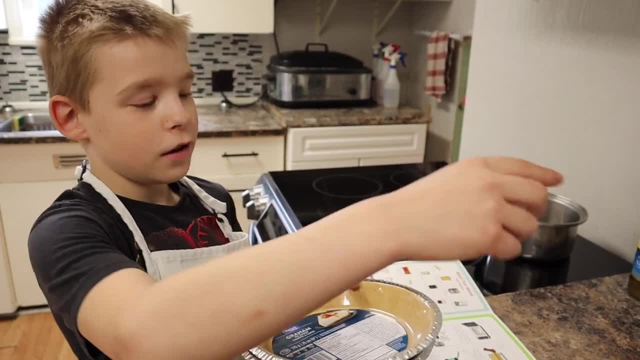 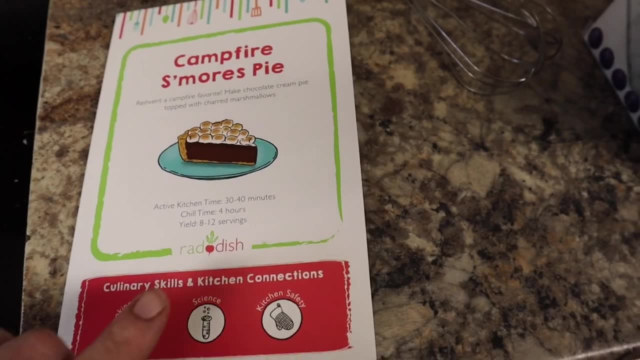 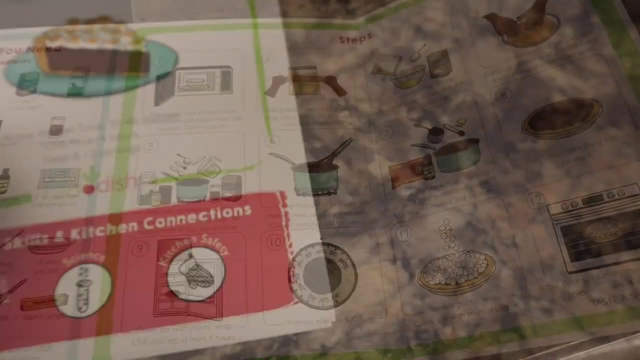 other three they can share because there's six and and four and four like that. So we are using radish recipes. We've had a subscription to this company probably for the last four years and I love their recipes. This is not a sponsored video. I just love their product. Their recipe cards are 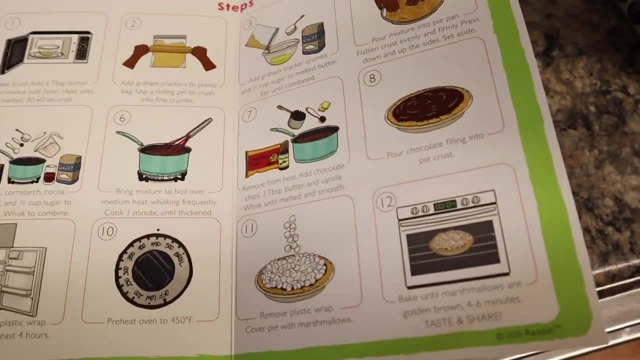 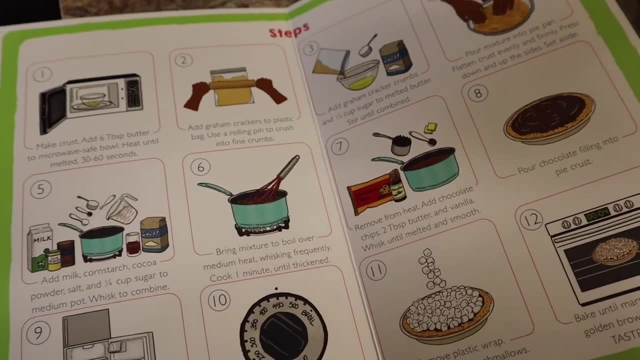 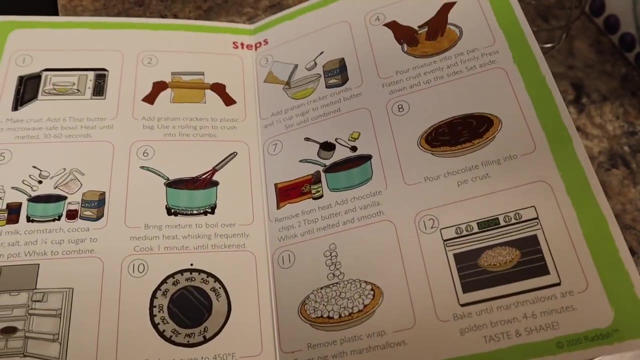 a plastic coated one. They have step-by-step directions. Their directions have pictures and then a brief description. They're very easy for the kids to follow. I would highly recommend this for anybody that needs a little bit of extra assistance when following a recipe. Do you like these kind of recipes? Yep, What do you like about them? 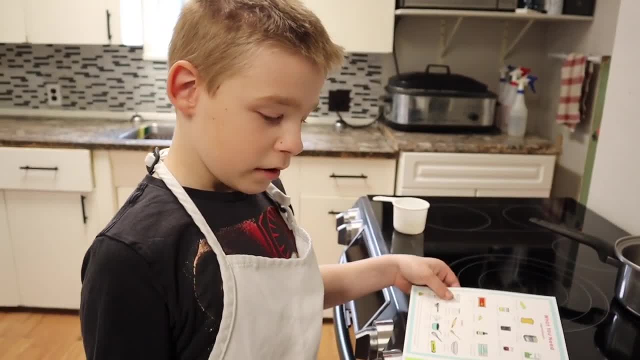 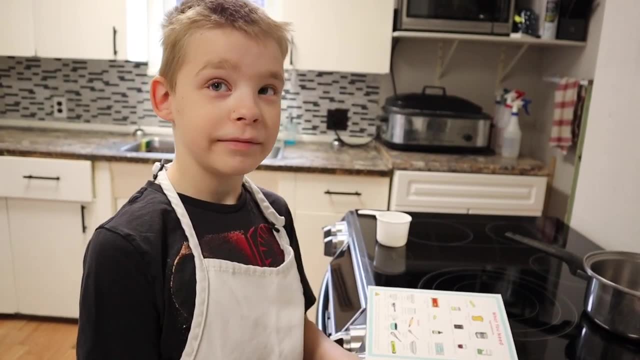 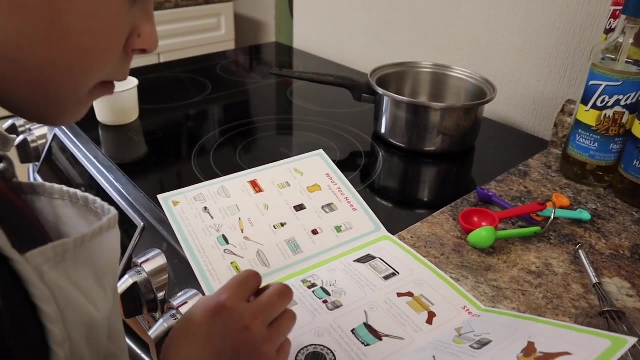 Um, they're. they're, when they're done, you um taste and share, and and they're so good when they're done That they have such good food. Yeah, Okay, What do you have to do? first, Add milk. How much milk do you need? Um, I have no idea. So remember, we look over here. 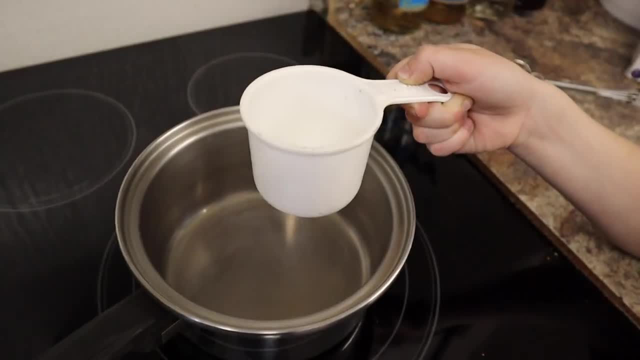 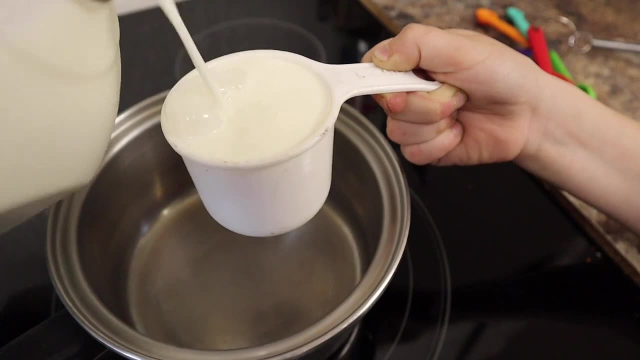 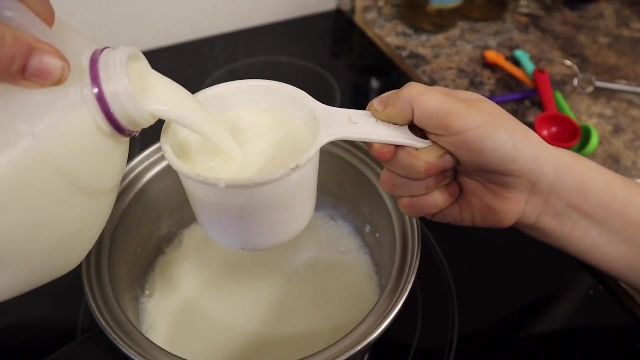 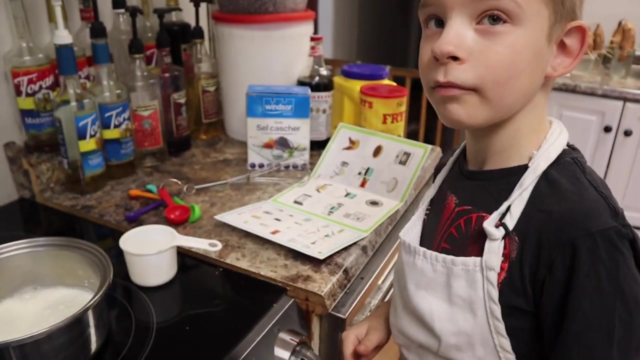 where the ingredients are Two cups milk. Okay, so it's a bit too heavy, so I'm going to help you pour. Yep One- Two. So, based Basically, we are making a chocolate pudding to go into this pie shell. Yep Three- cornstarch. 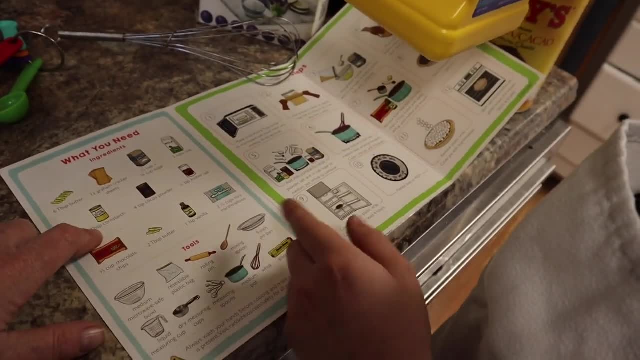 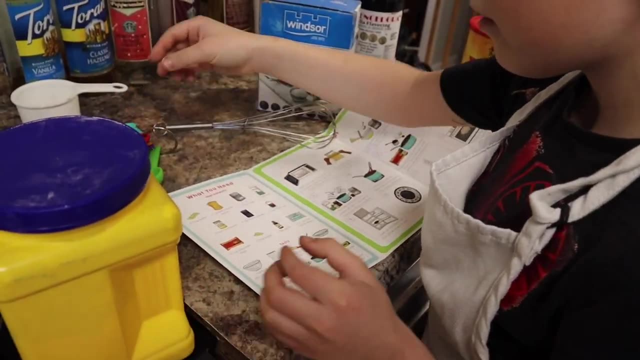 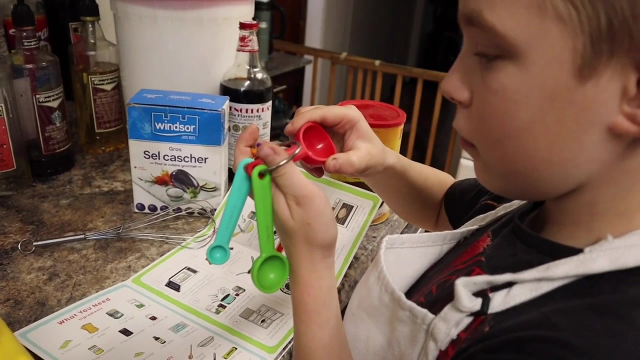 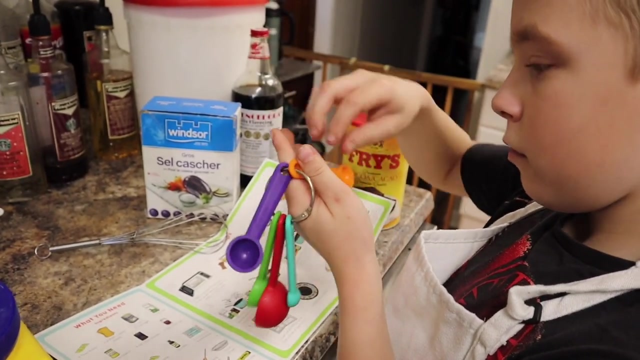 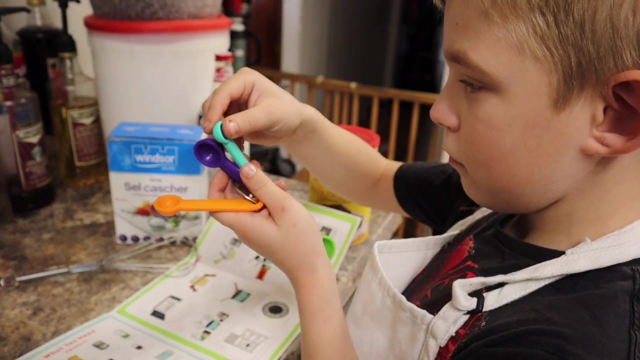 Three. what Cornstarch, What? what kind of measurement Tablespoon, Tablespoon. Three tablespoons Of this. Okay, let's do that. Which one's the tablespoon? These Find one that says tablespoon. None of them. None of them say tablespoon. 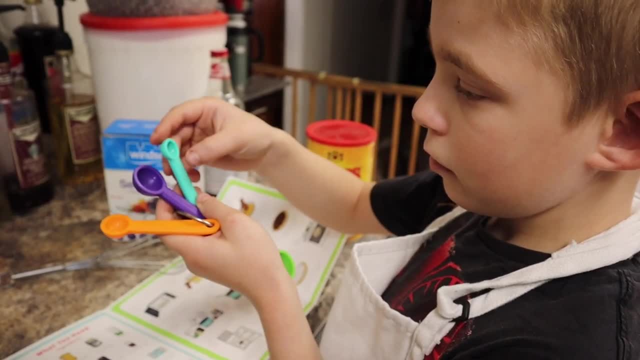 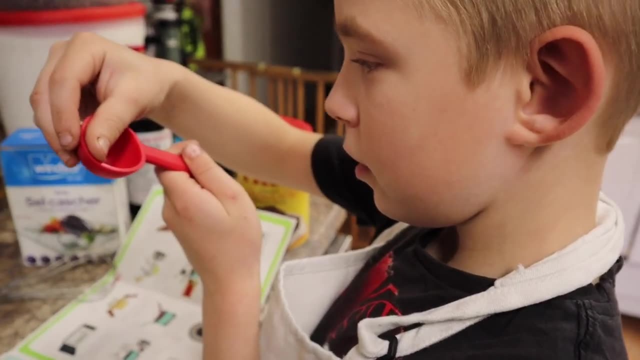 Tablespoon, Tablespoon, Teaspoon. I'll give you a hint: It's the biggest one, So this one. So does it say tablespoon on there, T-B-S-P. Is that the same as this, The abbreviation? 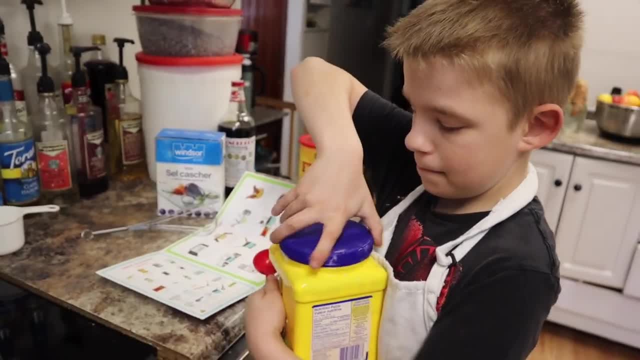 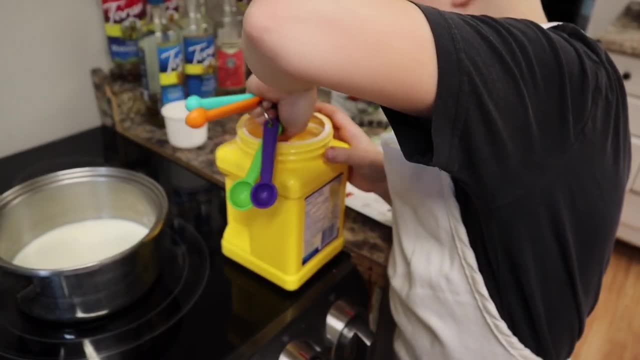 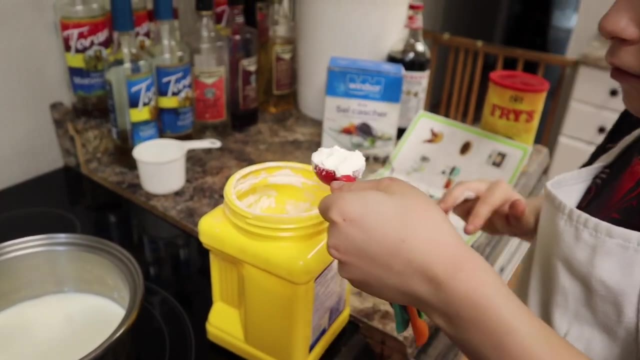 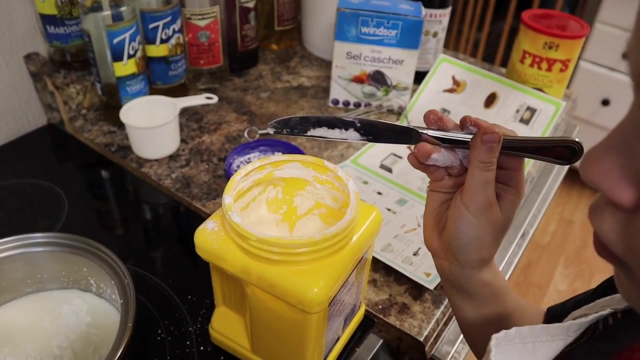 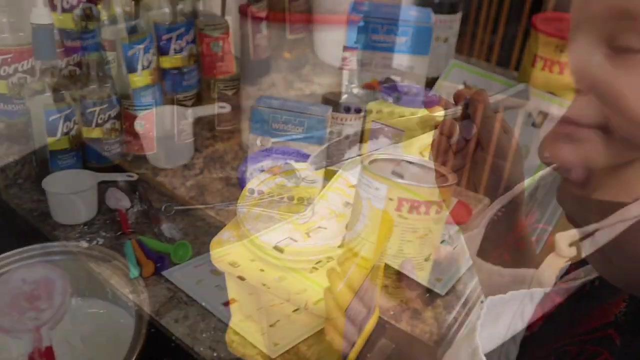 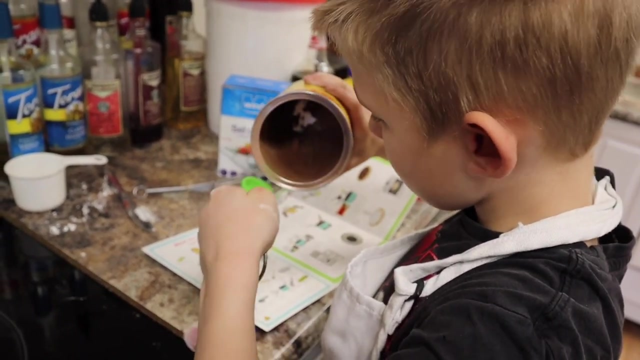 Yeah, Make sure it's nice and flat on the top. Okay, would it be better to use a flat knife than your fingers? Oh, okay, Nice work. Two, Three. Cocoa powder: Yep, How much of that are you putting in? I think you're gonna have to scoop it. 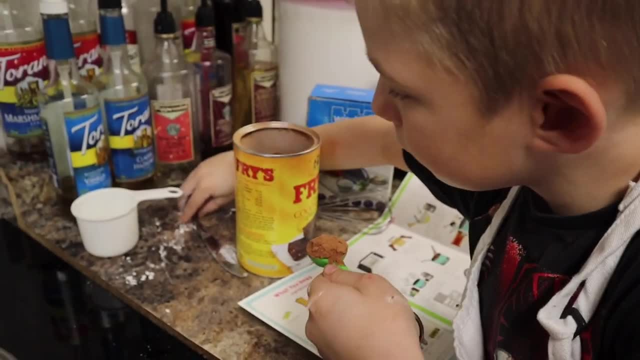 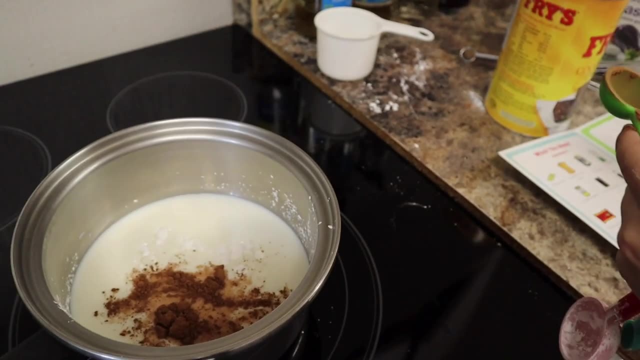 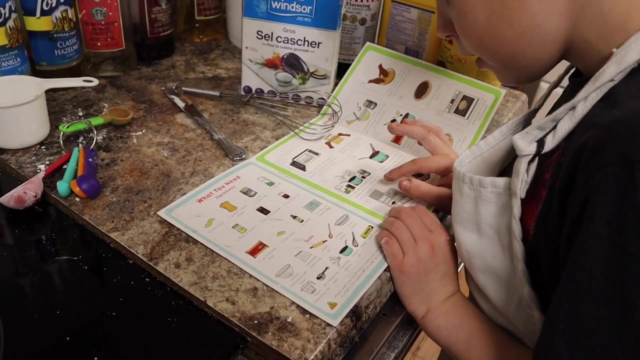 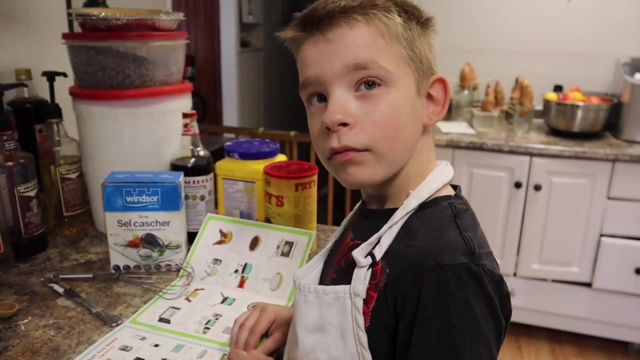 That Is it flat on top Me too. Otherwise it's not the right measurement. One: You need four, Four of those. Next, we need salt. Okay, so remember with salt what happens if you accidentally put too much in: It'll taste weird. 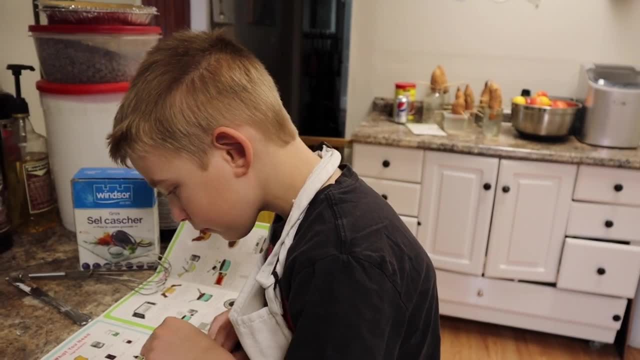 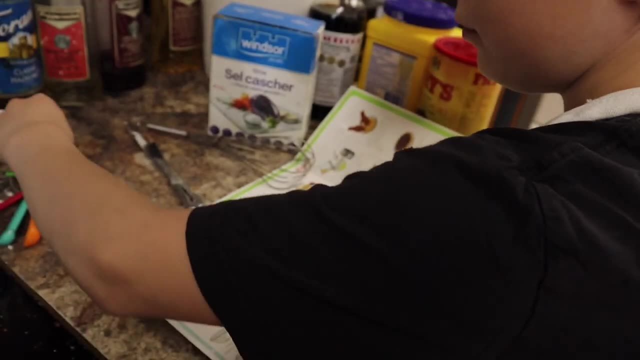 Okay. so we have to be super careful when we're putting the salt in that we get the right amount. Ah, 1.4 teaspoon, A quarter of a teaspoon. So this one, That's a full teaspoon. This one Does that say a quarter. 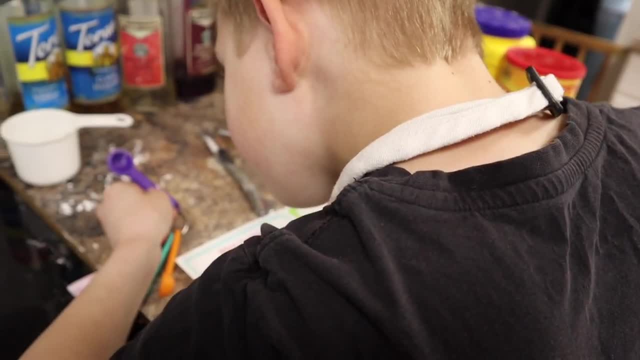 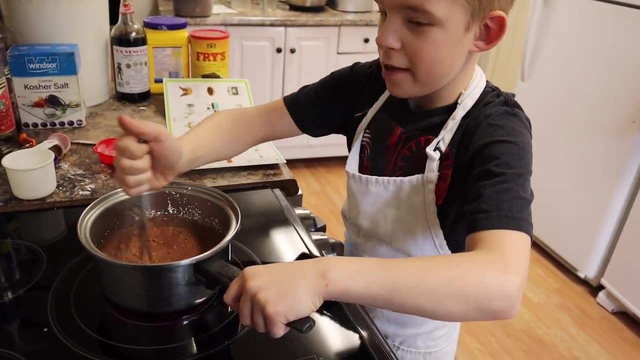 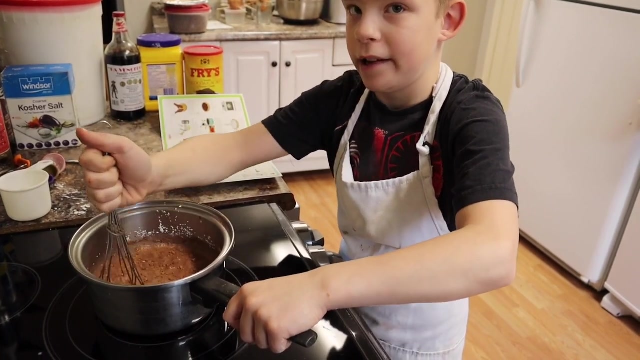 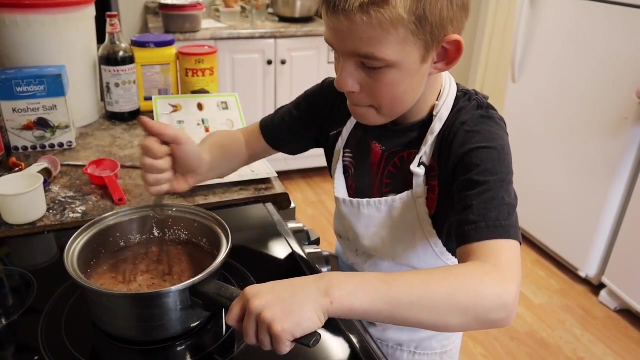 One and a half. So you're gonna whisk this all together, Yep, And you're going to bring it to the boil. For how long does it have to boil? One minute, And then it'll thicken up, Yep, Like that Is it all nice and smooth. You don't want chunks in your pudding. 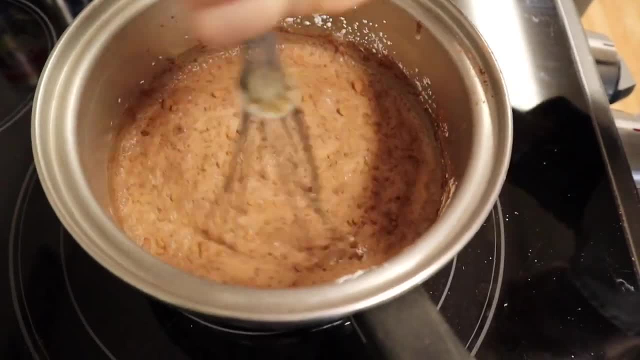 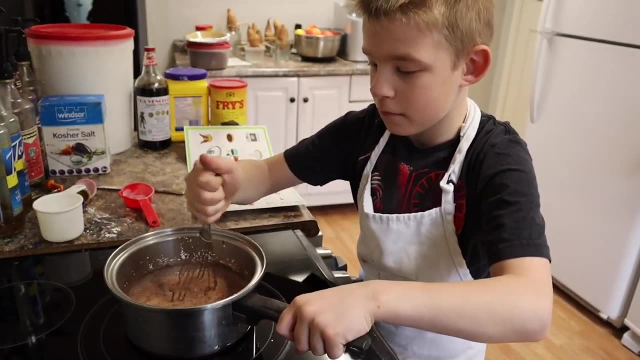 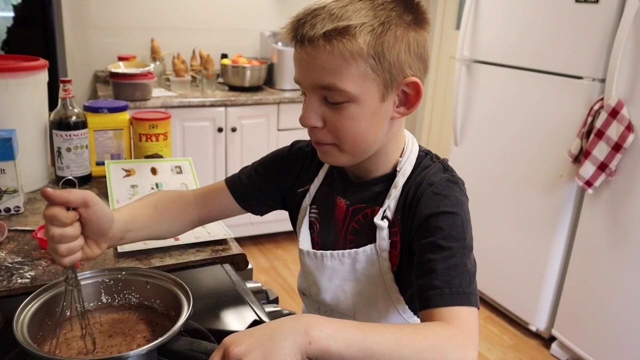 Nope, The pudding will be delicious. Right, I think it will be. We haven't made this recipe before. Good thing I picked it. It is a good thing, And I have a taste tester. Do you like to cook a lot? Yeah, 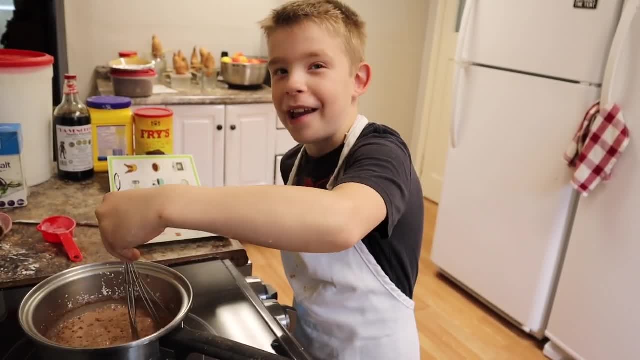 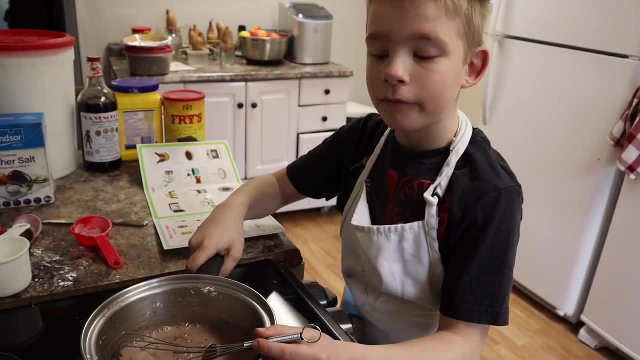 Would you want to cook dinner every day? Yeah, Or would you get tired of cooking? I wouldn't get tired. So do you know that If you didn't put the cornstarch in or the salt, you would have made chocolate milk? 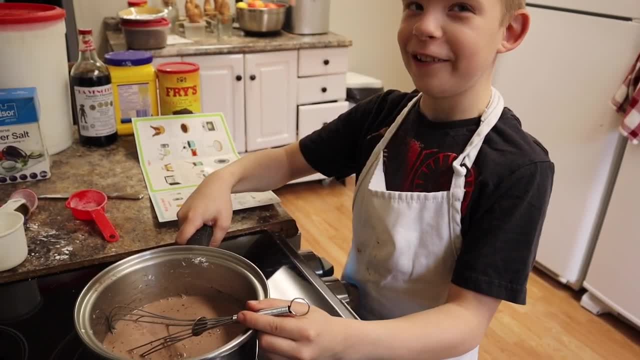 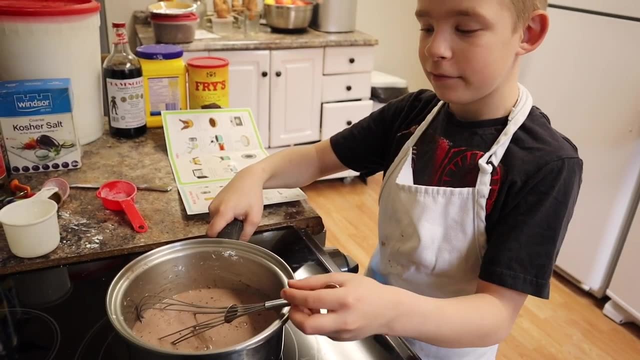 You know that you made chocolate milk. No, You could have had chocolate milk, but you're making pudding. Okay, You have to keep stirring because it burns easily. We don't want it to burn, And you have to stir all the way to the bottom. 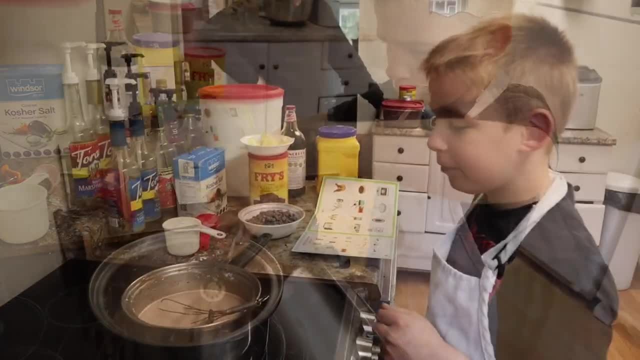 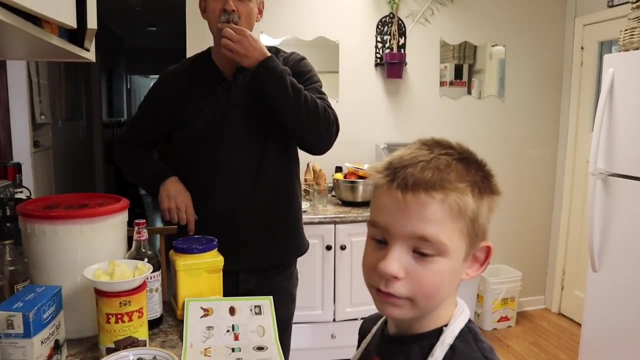 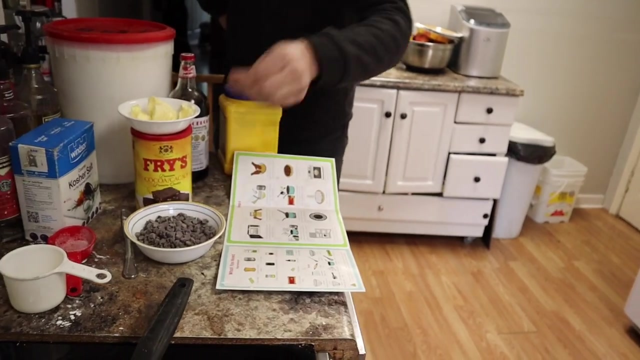 Yeah, it has to be all the way in. Is Dad coming to see what he can take? No, I think it is going to take What is Mum filming over there? No, Well, look again, See what Mum is filming over there. 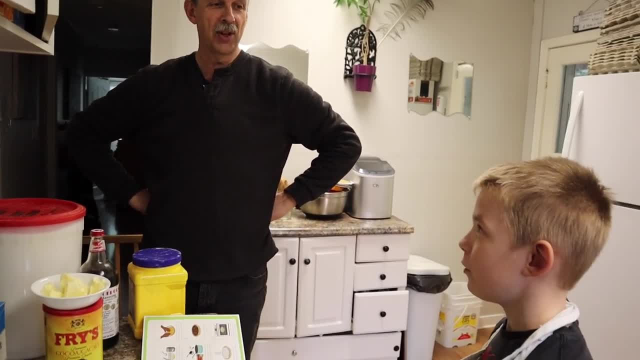 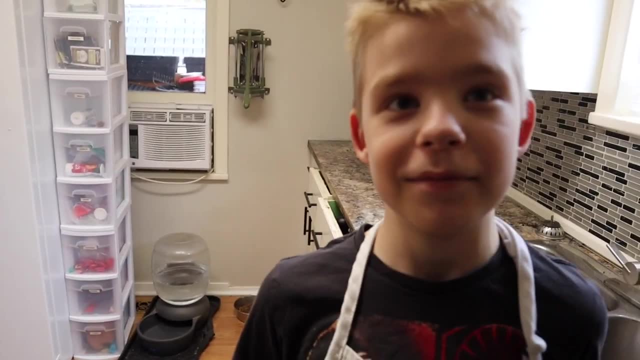 Um, Chocolate chips? I don't know. I thought she was filming something over there, I don't know. Look, Oh my gosh, I'm so done. Yeah, I love it. Luke, you're gonna run out of chocolate chips. Did you replace what he took? Yep. 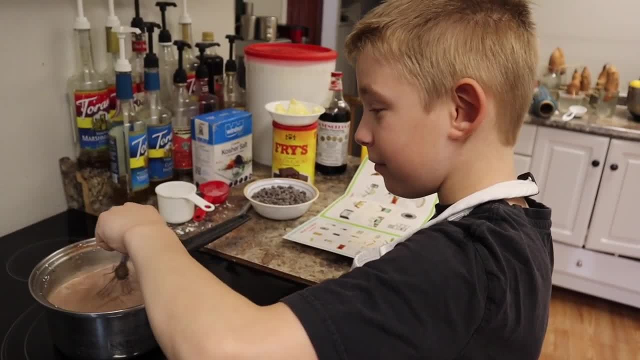 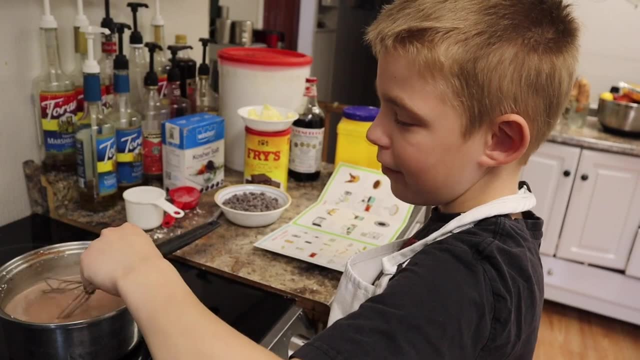 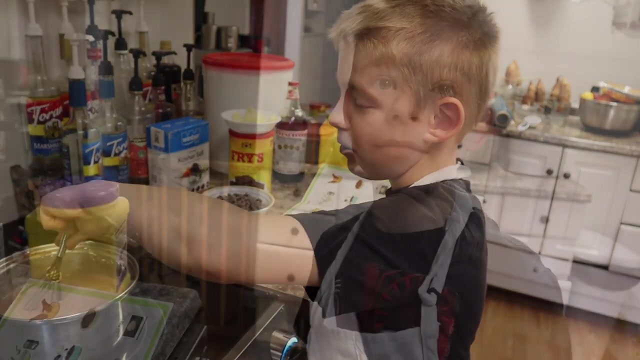 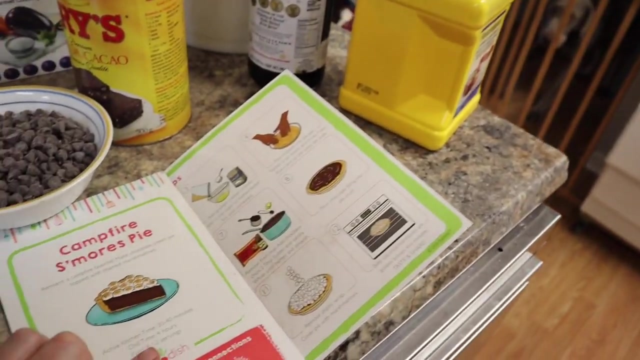 handful. Does he just come and steal all your cooking? Yeah, You need to cook things he doesn't like, Like he likes everything. You're gonna need a guard. This recipe says that a nine-inch pie- which is what you're making- will feed eight to. 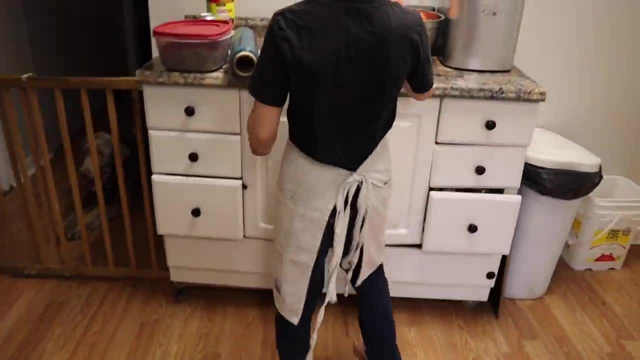 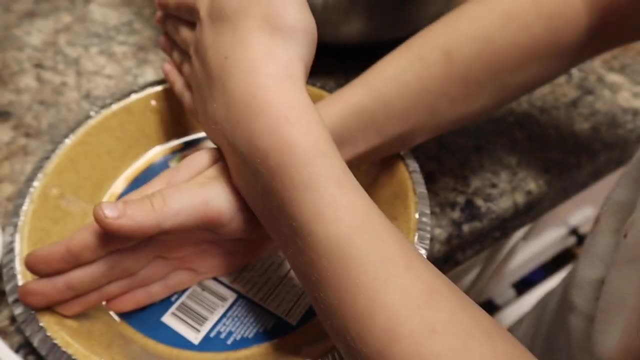 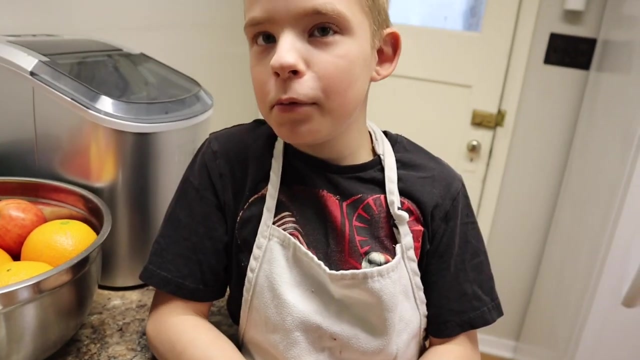 twelve people. If you come here, if you cut it like that when it's done, see, it'll go like that, But then you have to cut that into three more, But then then it would be too tiny, Then it would be too tiny. 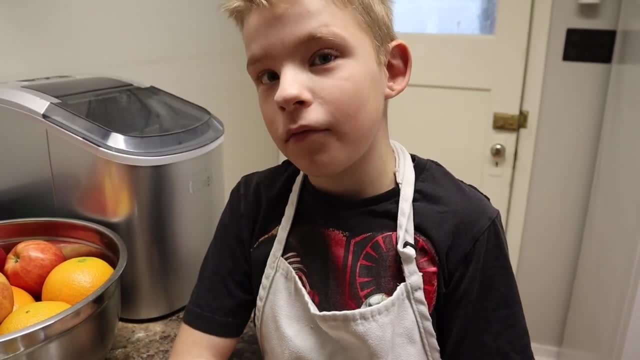 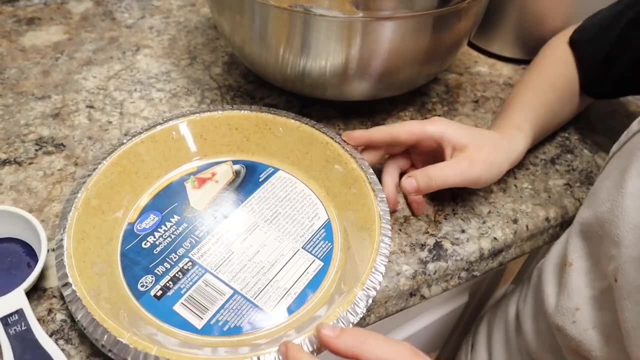 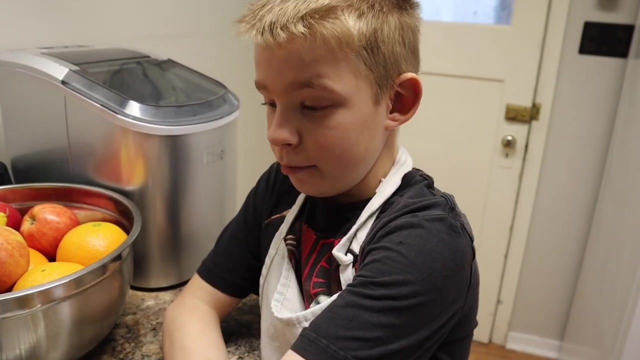 Okay, So you're gonna make enough pie for sixteen to twenty-four people, and there will just be nine of us, Like four, eight, then one more. You think you need one more? Yeah, two. So do you think the people watching agree with you or not? 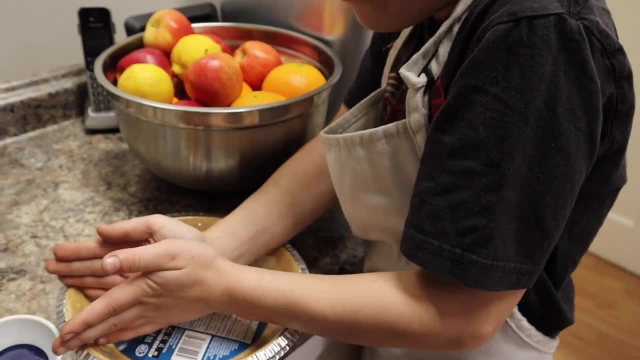 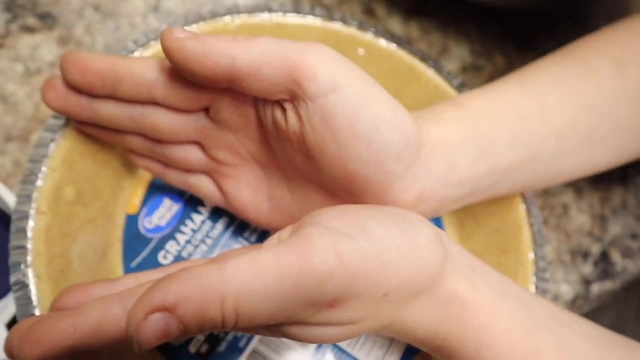 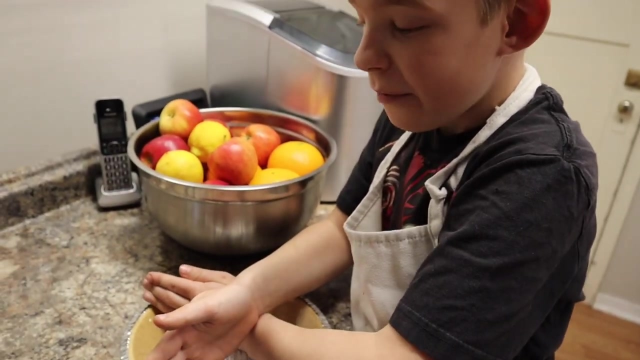 Because this see how tiny one little serving will be. That tiny, That tiny. Yes, Okay, leave us a comment down below if you think Luke is right. What if you have it? this big Perfect, You got the butter in. Can you put the chocolate chips in while? 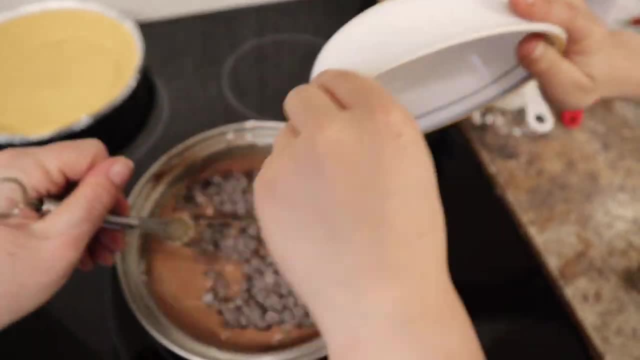 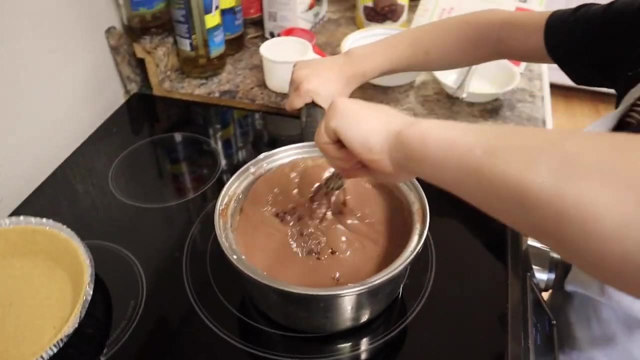 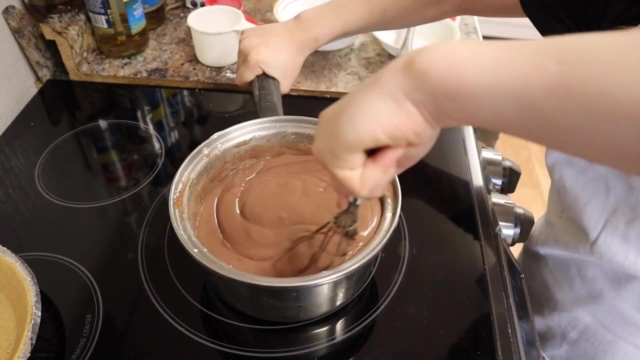 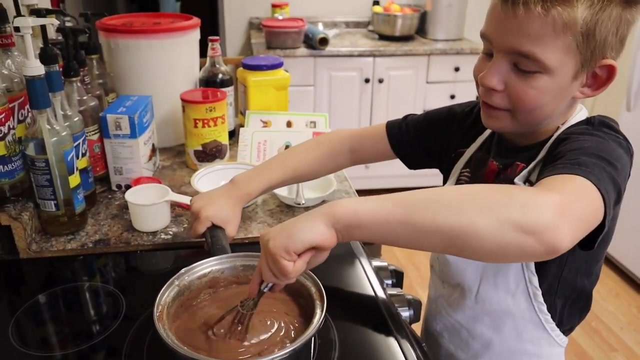 I stir it for you. Yep, There it is Okay. now you need to stir this in. Oh, Don't splash it out, Okay, Or it will burn. Mm-hmm, go slowly. so you need to melt all those chocolate chips. they already melted a little. good day, okay. 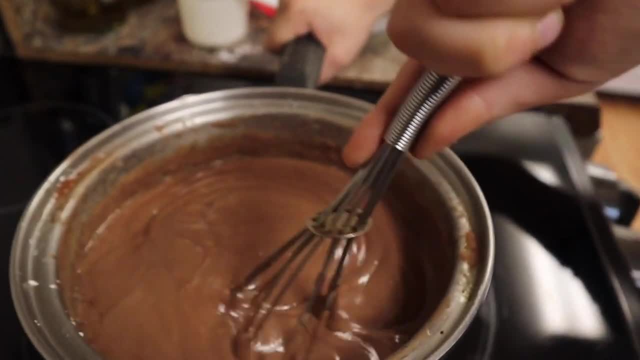 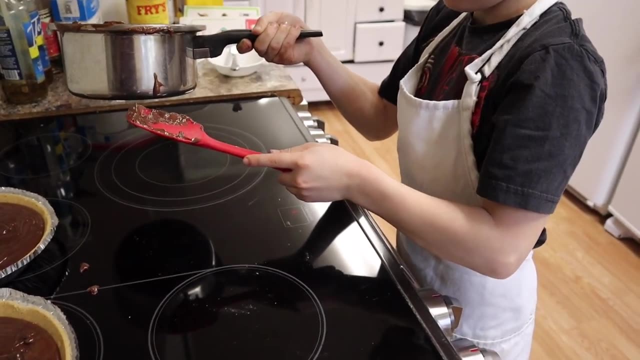 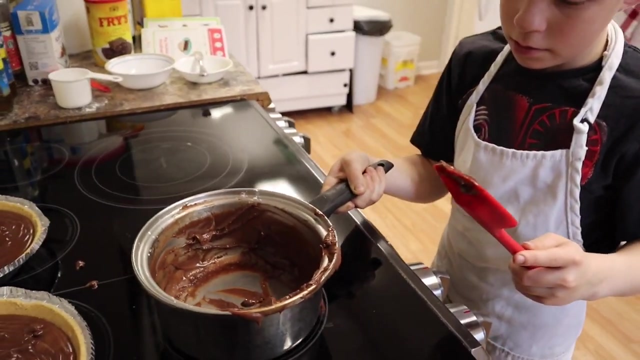 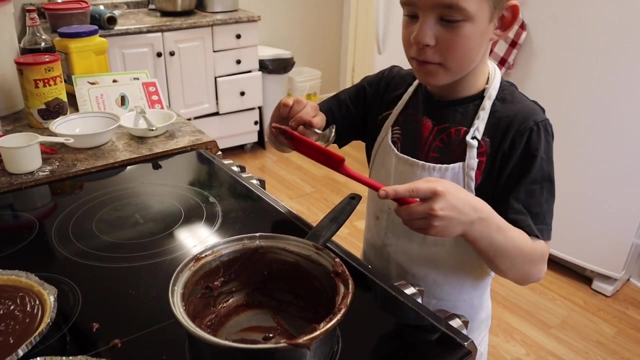 keep stirring. it's looking good. well, don't put it on the element because it'll burn. maybe you want to get a spoon put it. let's hear where it's not hot. maybe you want to get a spoon and taste it. mmm, is it any good? 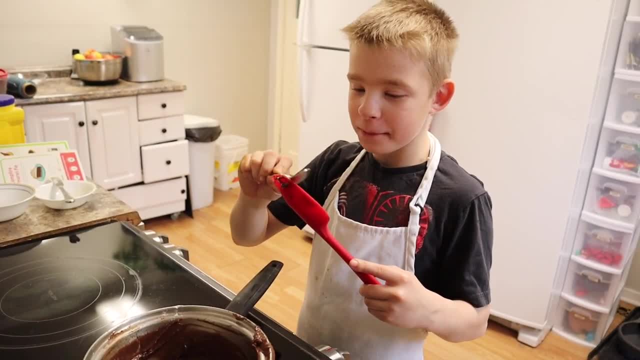 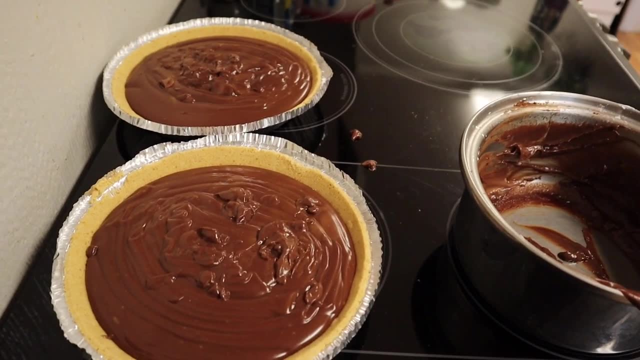 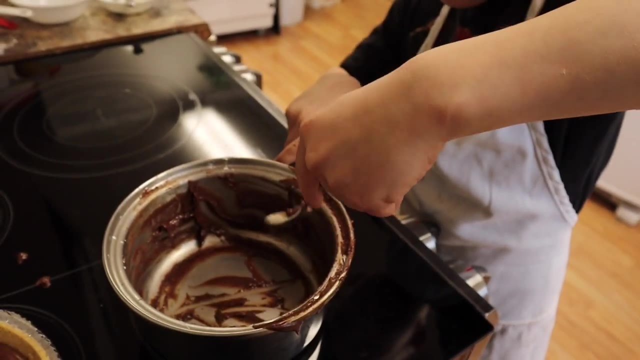 luscious, okay, and these pies, we have to put plastic wrap on it so that they don't get a skin on them. hmm, okay, is this the reason you like to be in the kitchen? because you like to be eating sometimes. sometimes fun making new things, isn't it? yeah, you're making me hungry. 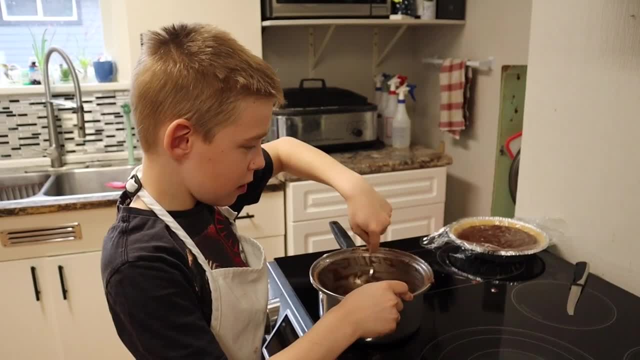 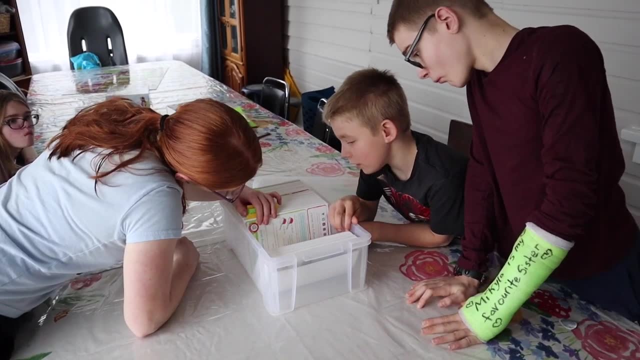 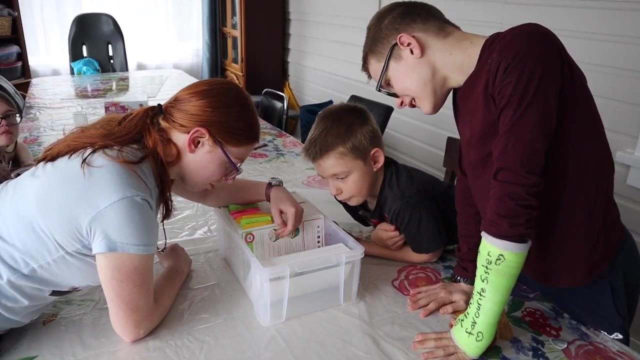 can i have some? okay, i'm just scraping it up. i don't think there's anything left. yeah, what does that say? orange blossom tea cakes- great, cupcake, cupcake. what is this doing? look at the different recipes. that way, when it comes to my turn, i can have an idea what i want to make. 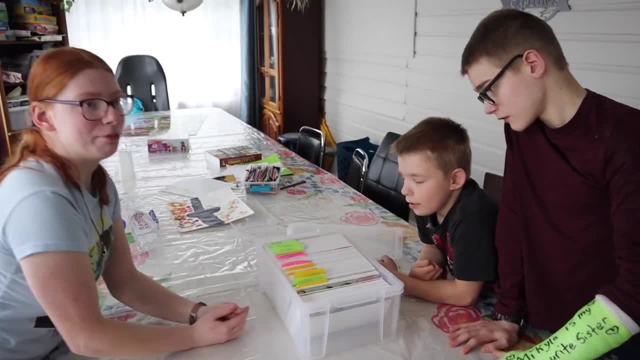 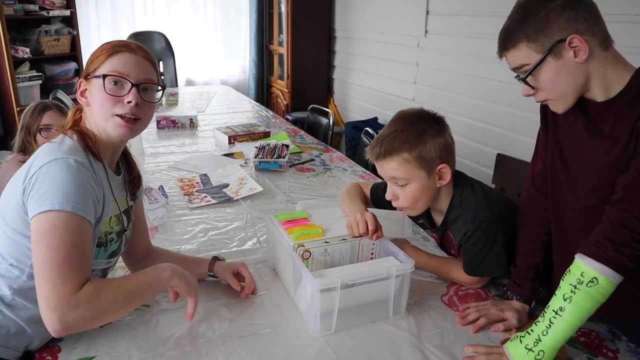 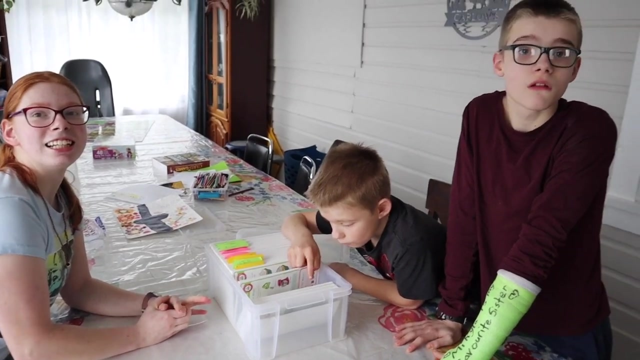 what do you think you want to make? i want to make since one time which, when school was in doing indoor school, we made these circular like pizza cake things, the cake pan. i thought pull apart pizza stuff. yeah, that nice. what do you think you want to make? um, either chinese fruit or 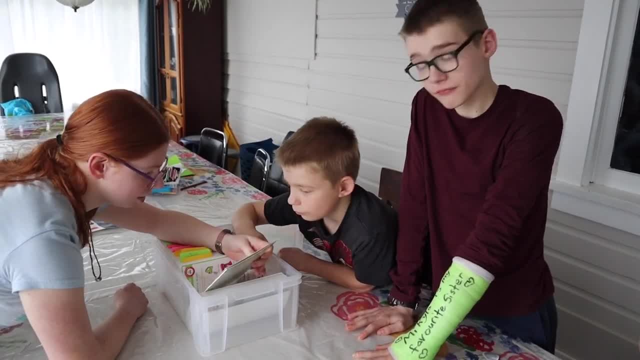 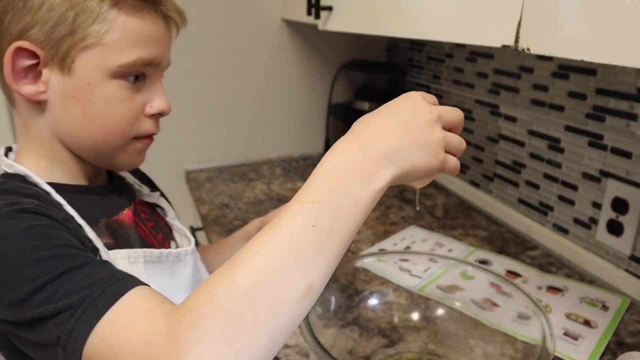 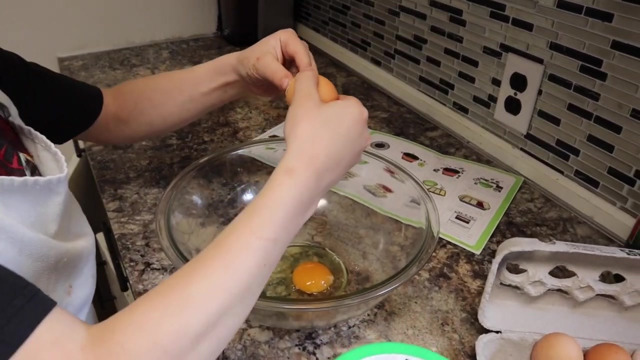 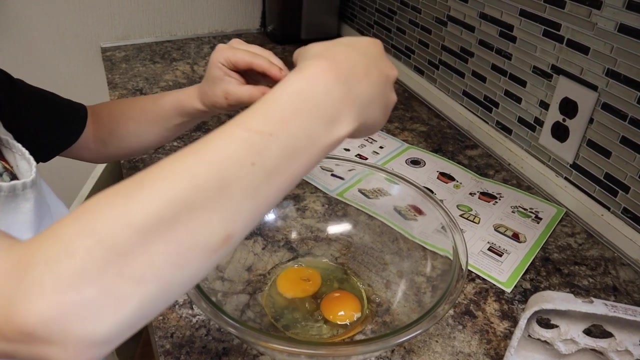 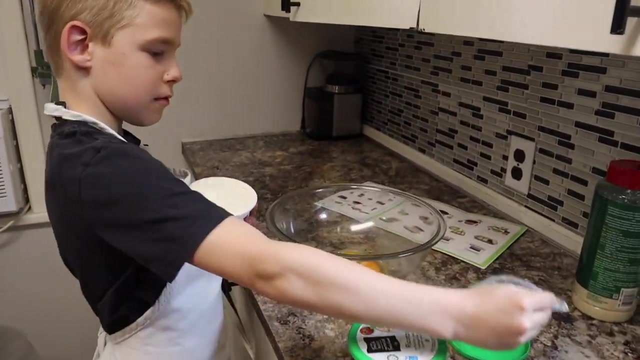 meal or pasta. this is good. have some. it is how come she is getting the ар. wouldn't have it done, but we have to do it now. we love pizza. What is it? Ricotta, Ricotta cheese. Yep, So you're making the filling for your. 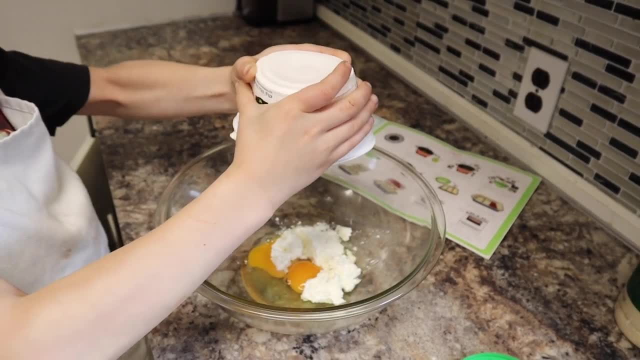 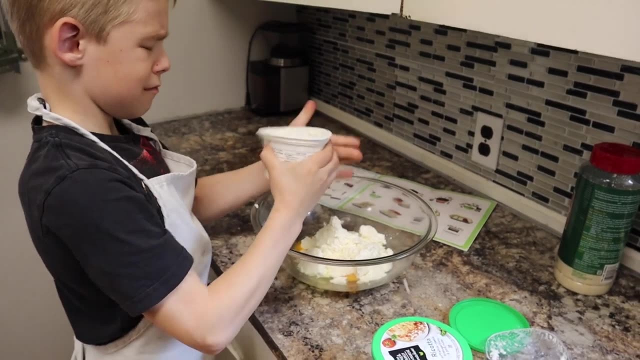 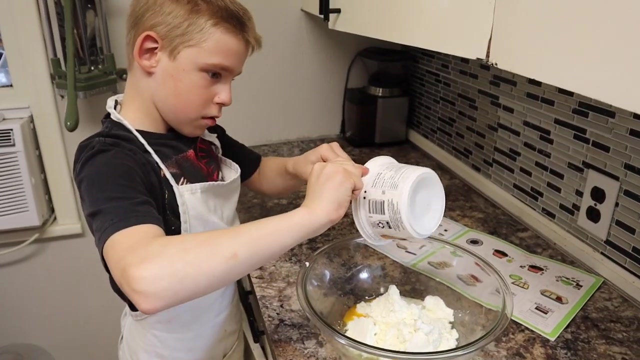 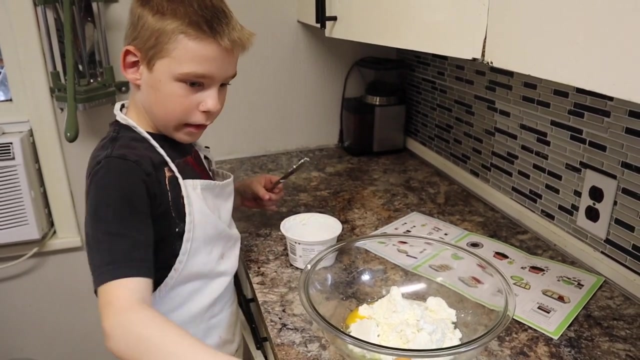 lasagna? Mm-hmm, You might need to get a spatula. So do you think your adult siblings aren't coming because they know you're cooking? Yeah, I think no. Is that what? are they scared because you're? 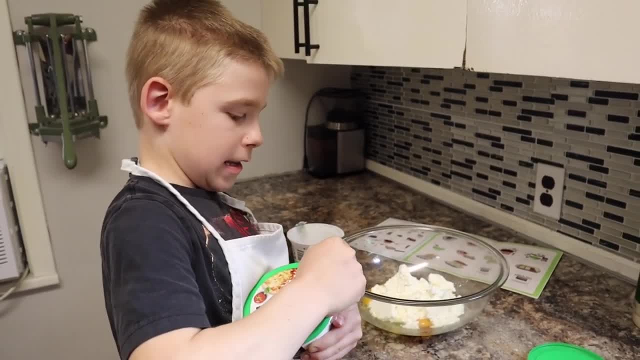 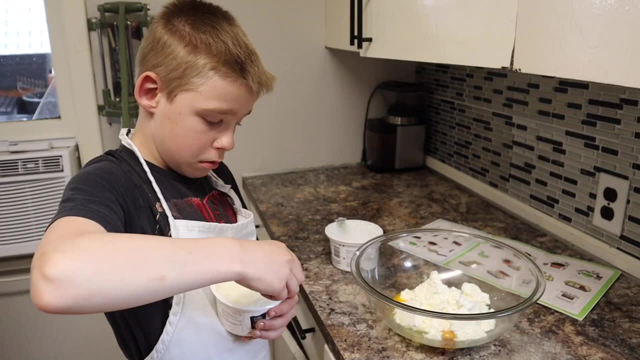 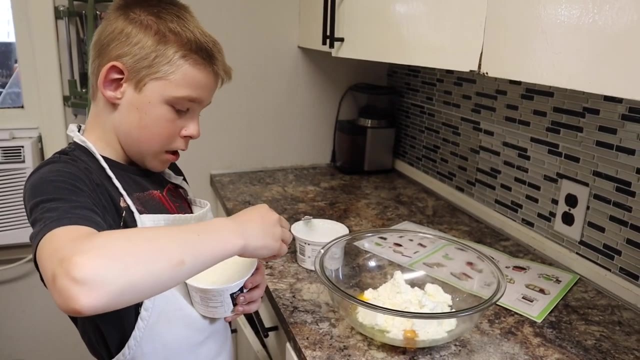 cooking. No, because, because, because Aaron is not sick And they went to yourselves, You got the wrong one. Jay's sick. Yeah, Jay, So that's why he's not coming. Mm-hmm, No, so I decided to not to. Oh, I thought it was because you. 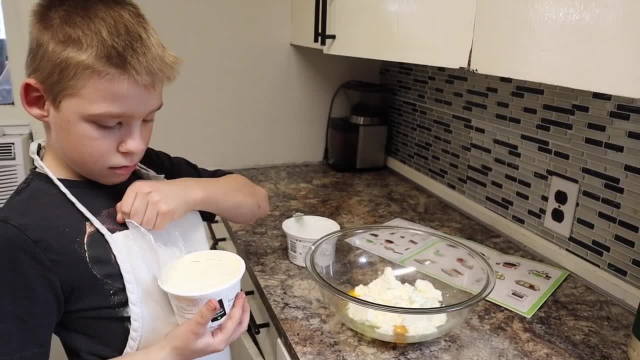 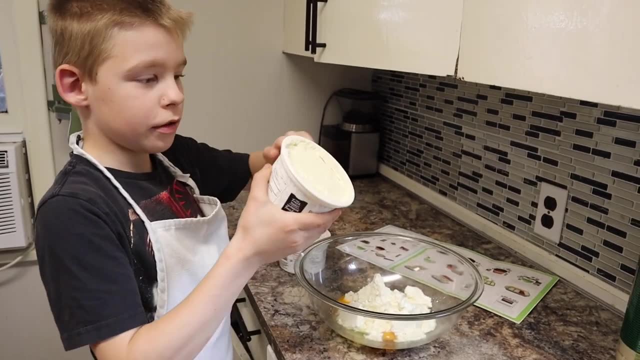 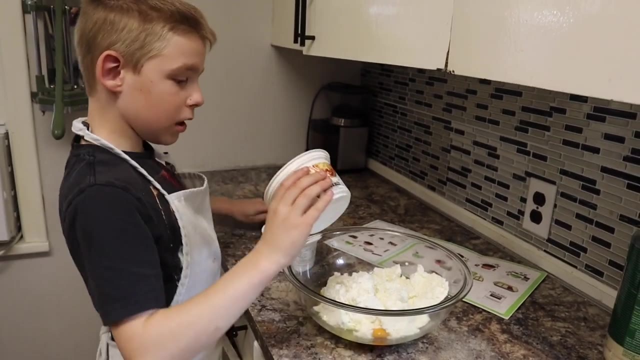 were cooking and they were scared. No, Are you a good cook? Yeah, How good Good. The best cook ever. All this? This too, Yes, please, The best cook ever? Not really, But you're working on that, Uh-huh. 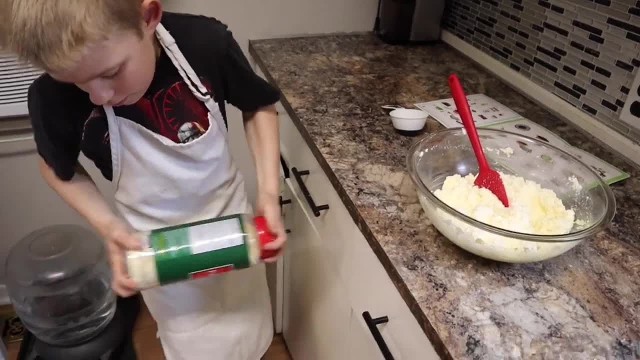 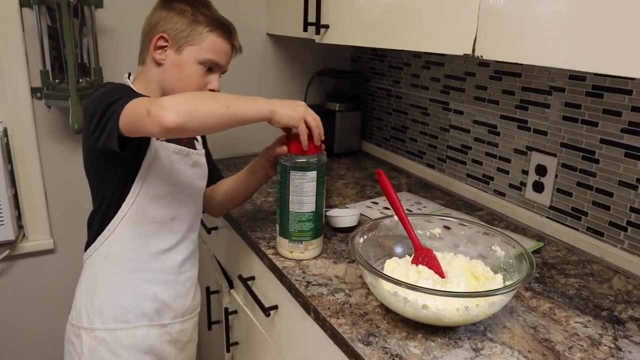 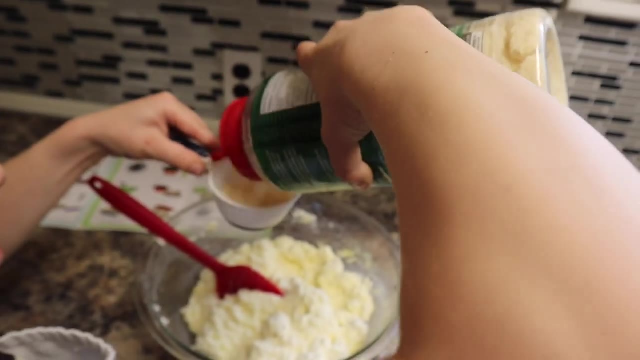 You're learning some new skills. Yep, What are you doing? I'm checking it because there's big chunks, Oh. So how much has to go in A full one of this? Half a cup, Half a cup, Yeah, that is half. 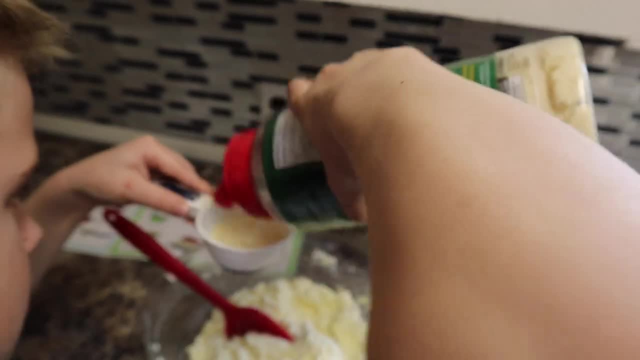 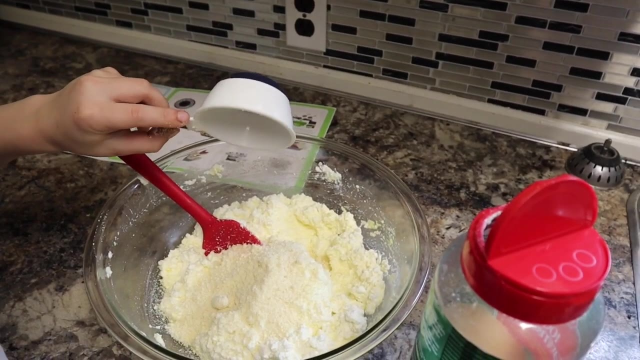 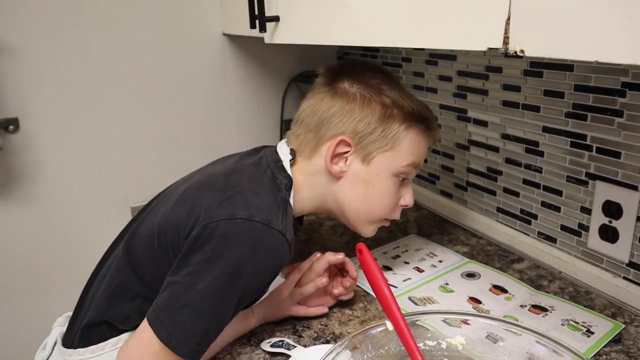 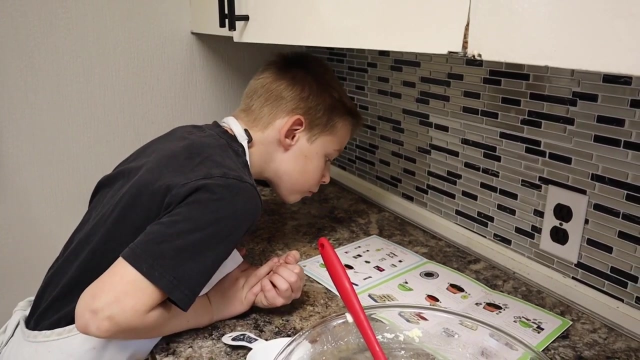 a cup, Nope, fill it right up. So you have half a cup of parmesan And don't Some ricotta cheese, Two eggs. What's next? Next you have to put pepper. How much pepper are you gonna put in there? Um pepper, Half, Like this. 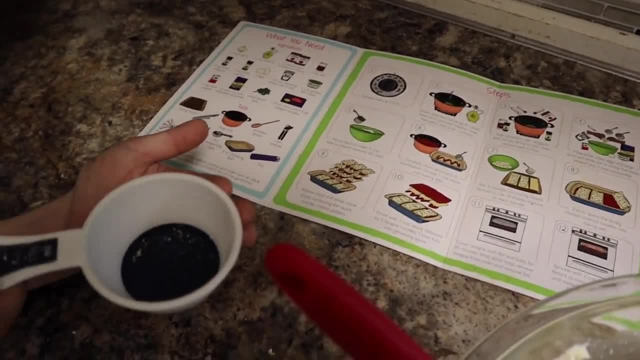 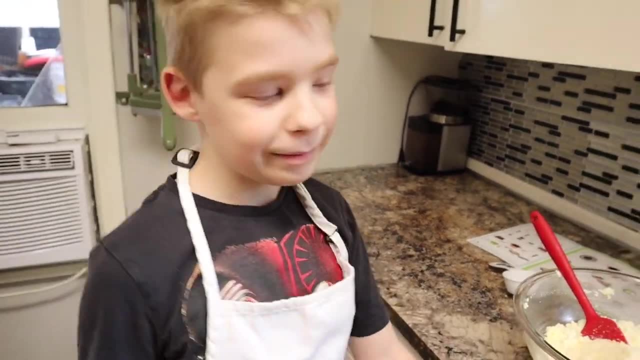 That's a lot of pepper. That's going to be super spicy. Do you think you are reading that wrong? Oh, a teaspoon. Oh, that's a big difference. You would be burning everybody's mouths off. How much is half a teaspoon? 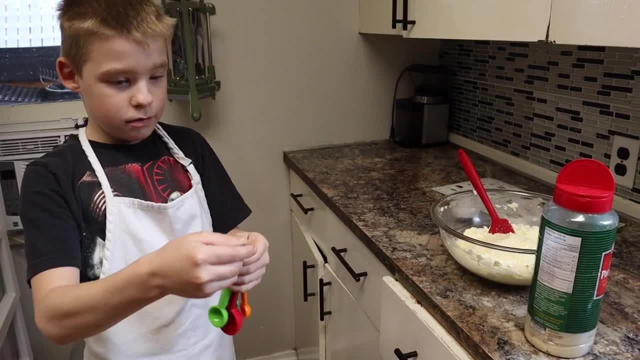 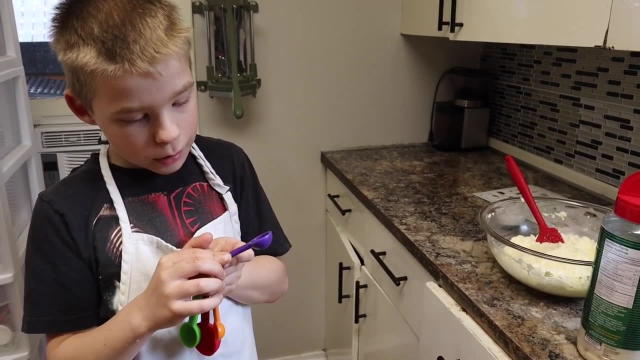 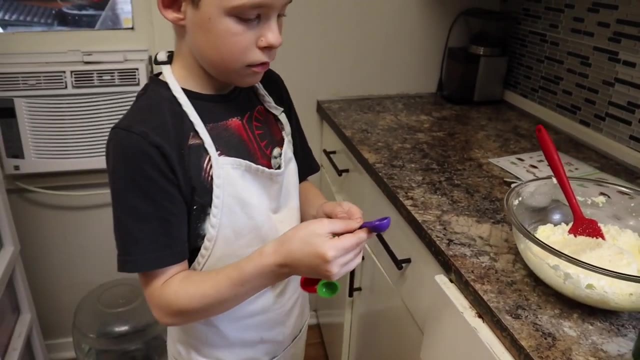 This? I don't think so. This one. What does it say? Are you reading it? Um, 1.2 teaspoons, 2.5 milliliters, One half, One half. So this Of pepper, That's a lot different than that cup full. 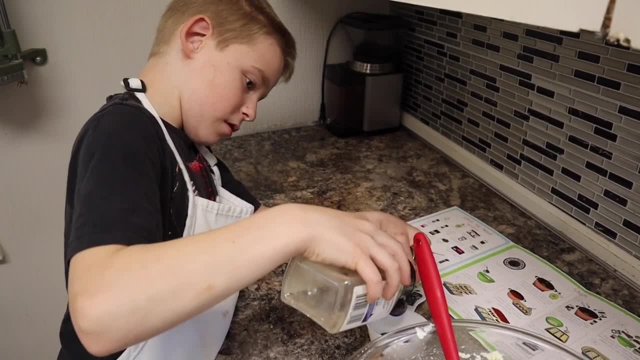 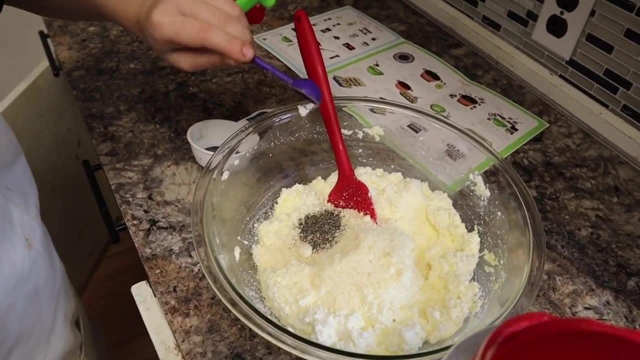 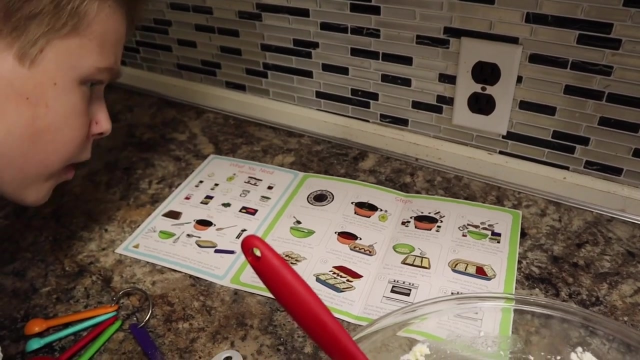 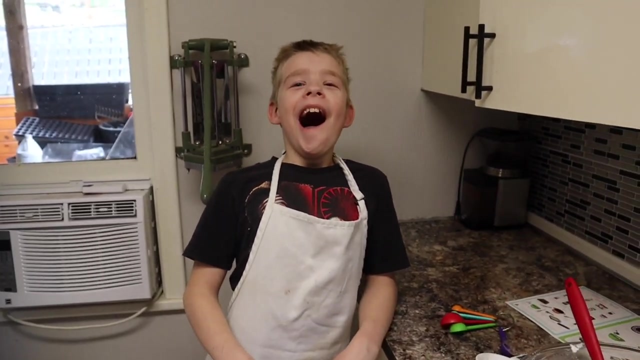 Yeah, Would your mouth be burning if you had put that much pepper in. I think so Wonderful. What else? This Next is two cups of Merzla. Of what Too much pepper? Oh no, Get away from the food. 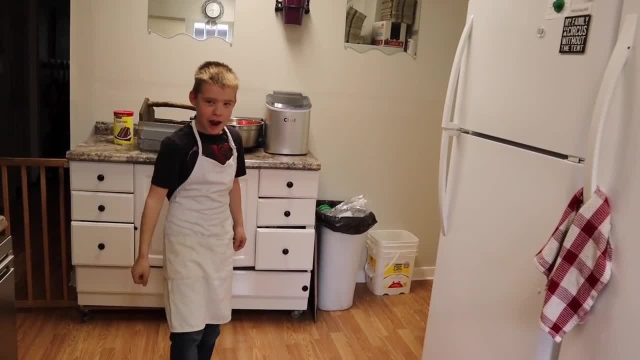 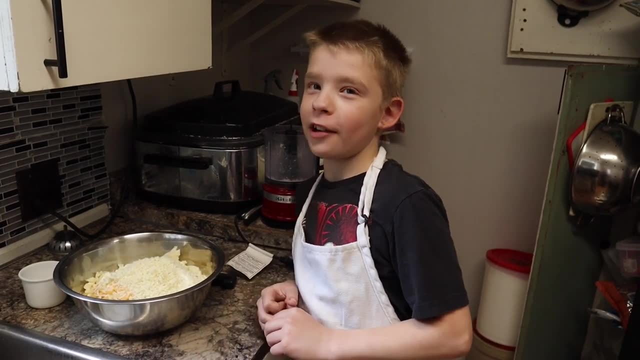 Oh, good thing you got away from our food. Pepper makes you sneeze Two cups of what, This, What is it? Merzla, Mozzarella, Mozzarella, Mozza, Mozza Cheese. So, because we couldn't find. 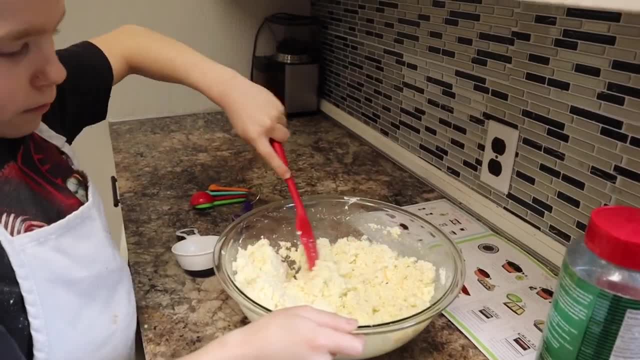 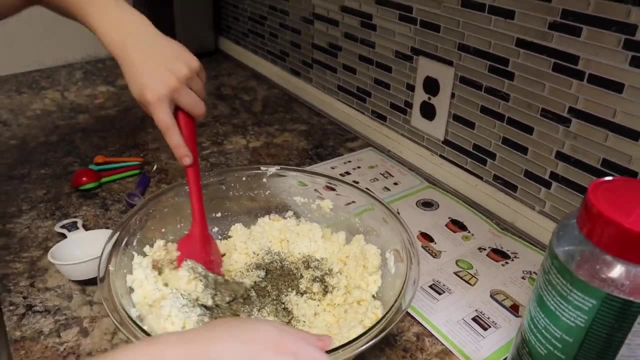 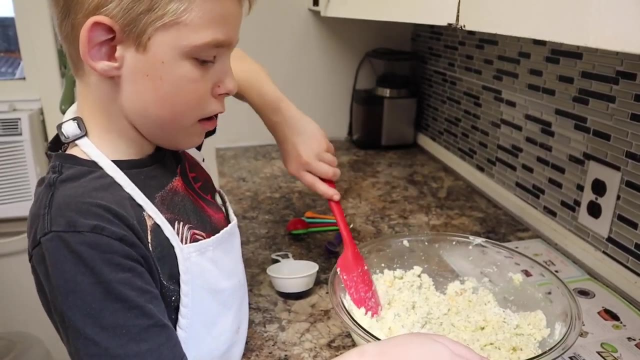 Fresh basil. you need to use the dried basil. Yeah, You know what? I'm just going to sprinkle some on. Stir it all in, please, And it'll taste, you know, good, Delicious, Yeah, Best dinner ever. 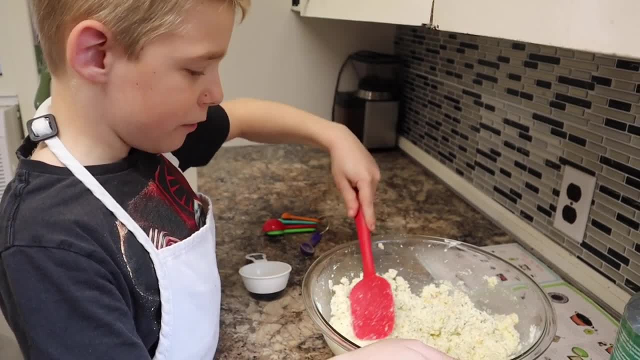 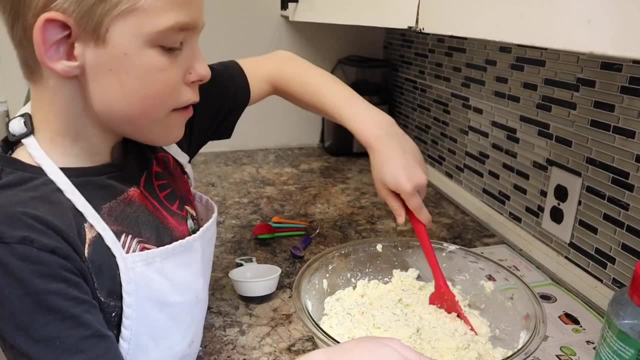 And then we'll have the pie to ourselves. Oh, so is that the plan? We're going to fill everybody up with other stuff and you and I are going to eat the pie? No, Everyone will have some too, but the adults are not here to eat it too. 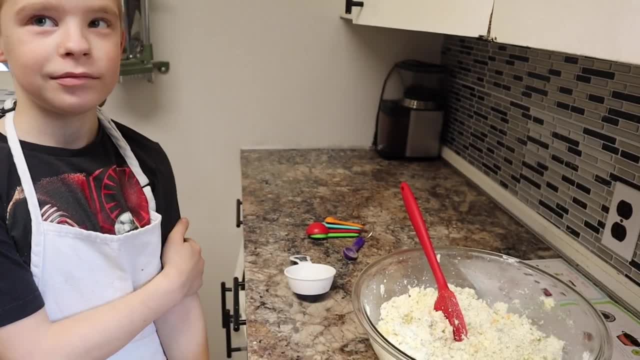 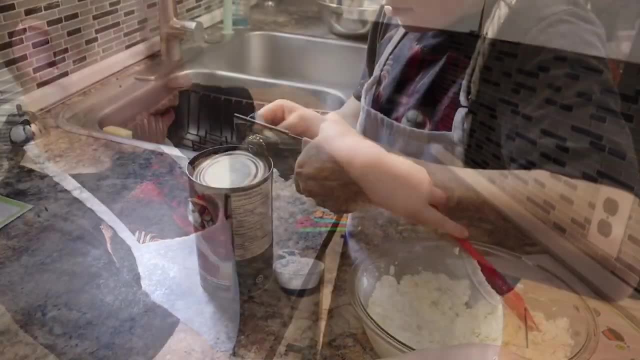 Oh, I thought just you and I were going to eat it all. If you want, We'll fill everybody up with this stuff, so they have no room for the pie. Yeah, So you decided to use spaghetti sauce instead of making your own sauce. 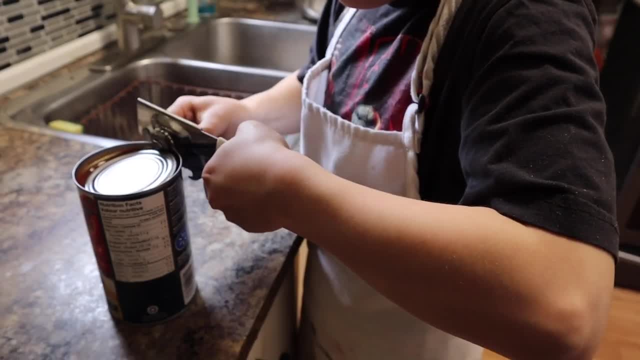 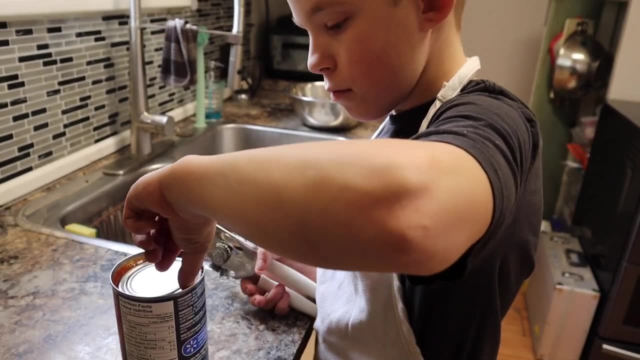 Yep, Do you think it's open? How many times are you going to spin it around? Just that one? Okay, open it up, Get it off of there. So another shortcut. Okay, be careful with that, because you could cut your fingers. 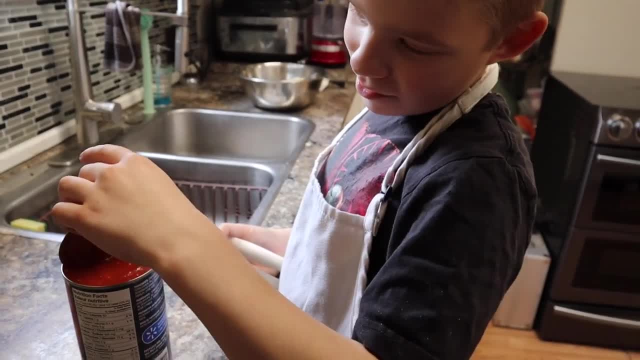 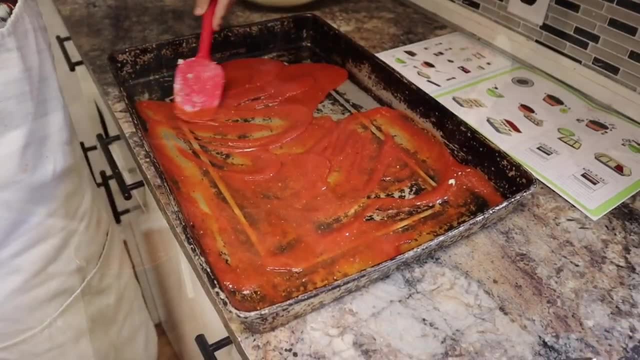 It's very sharp. I wasn't Well you know what. I thought I was being careful one time and I cut my finger and needed stitches doing that, So the sauce goes all over the bottom. Then we're going to start layering things. 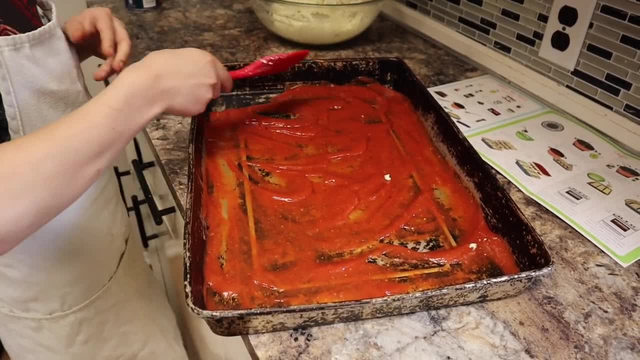 Hmm, How many layers of noodles do you think you're going to have? Probably three or two Or four, Probably Right. So these noodles are oven ready noodles, so we don't have to cook them first, Cool. So some noodles you have to cook ahead of time and others you can use them like this: 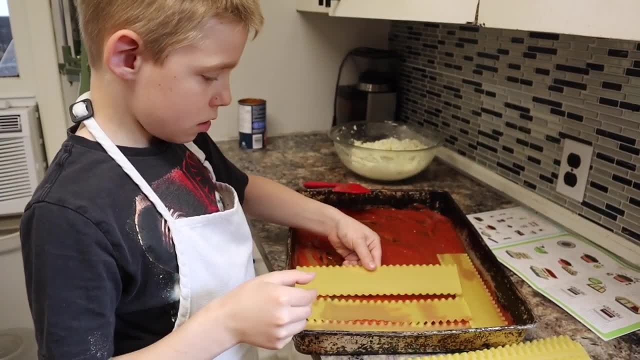 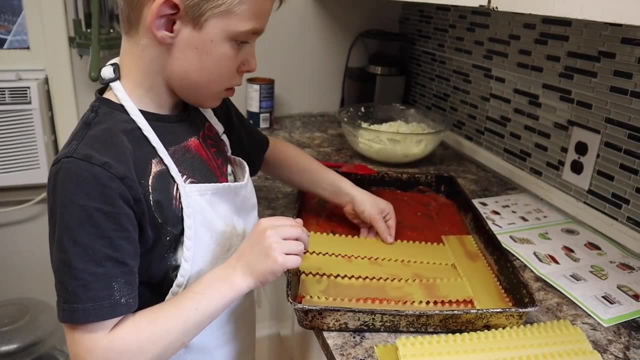 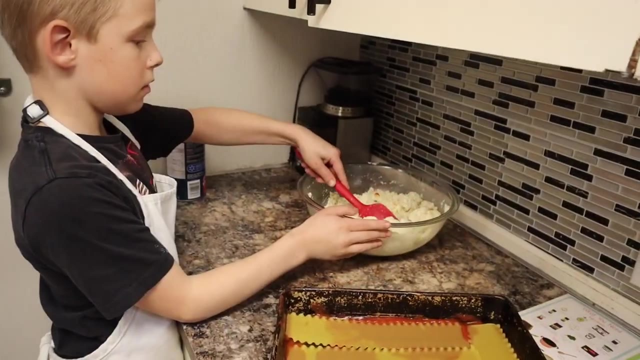 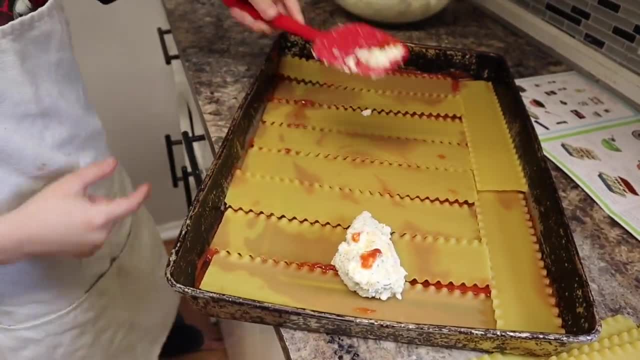 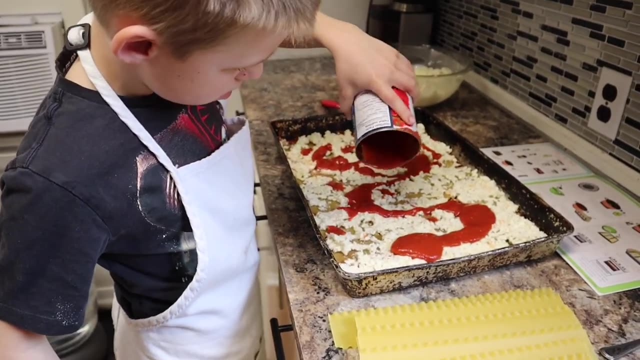 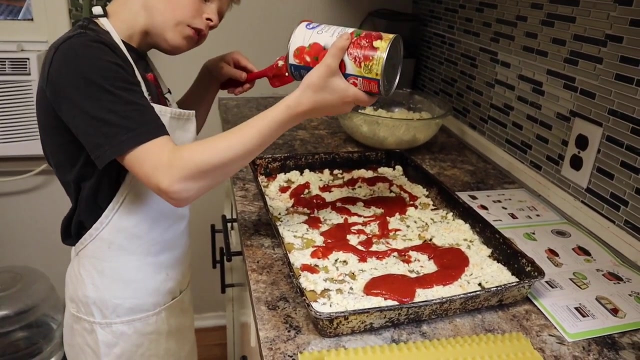 Okay, Okay, Okay, Okay, Okay, Okay. Next, you need some more sauce Like that. Well, you're going to have to spread it all around And we're just going to keep making layers. Huh, no more than that. 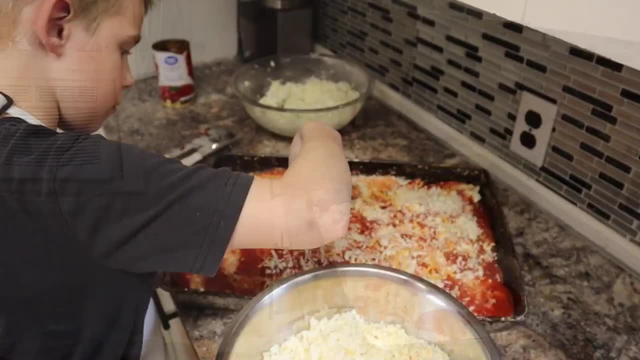 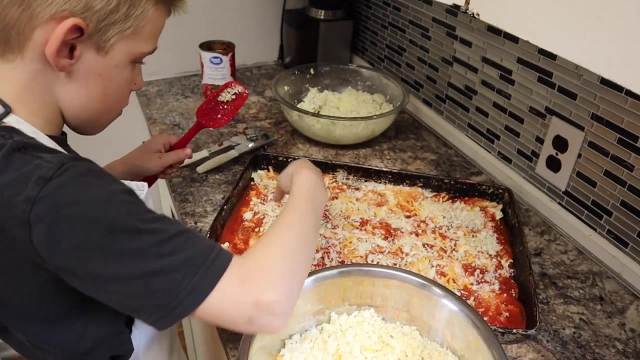 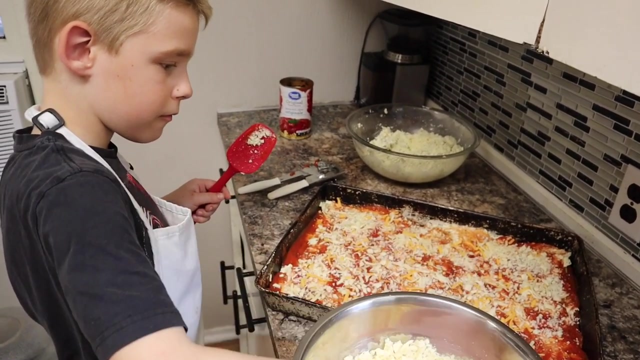 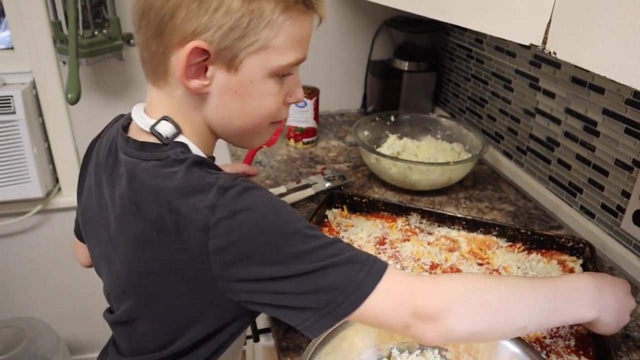 And I have to open another. can Yup, Sprinkle a bit of cheese and then we'll do a whole another layer again till the pan is full? do you think this will make us two dinners? I think so good. I don't want to cook tomorrow. I can cook for you. what are you gonna cook me? yeah, I can make. 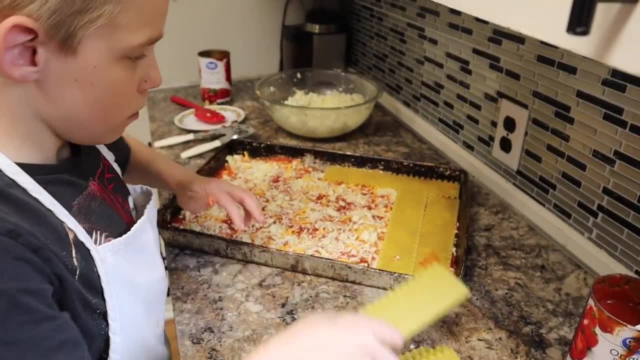 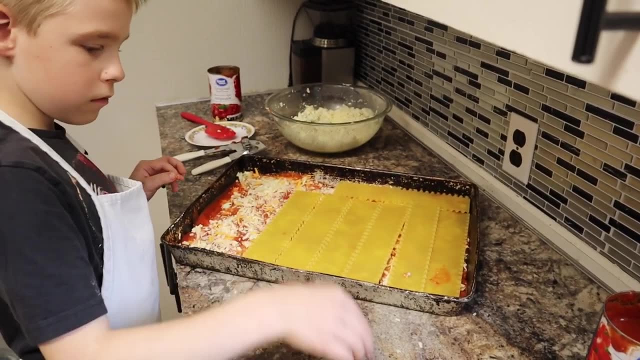 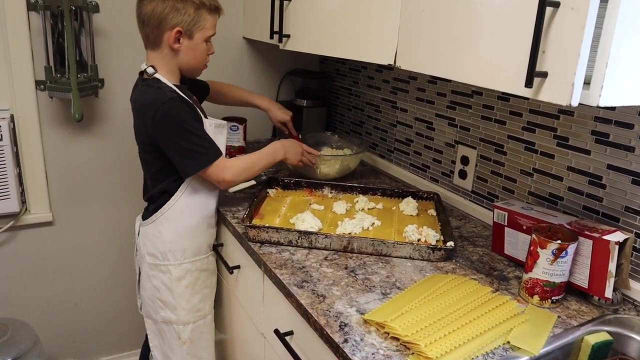 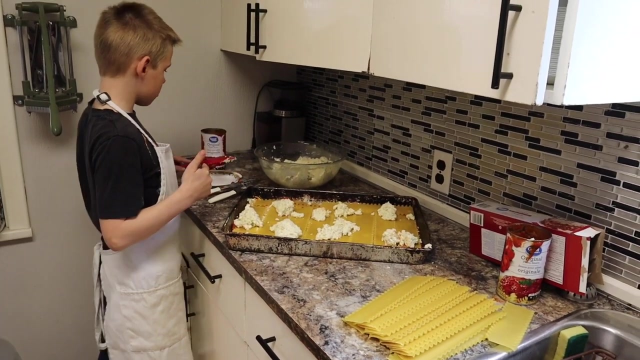 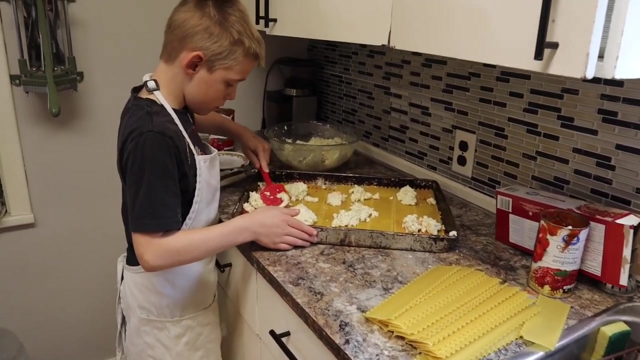 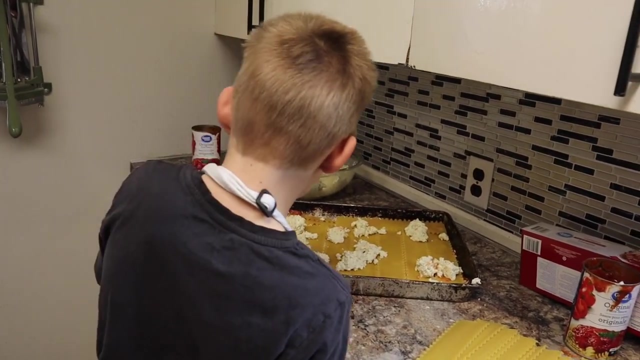 homemade pizza maybe? oh, I think so. now you need to spread it out place with what you could use that spatula, yes, do you think you want to be a chef when you grow up? to get to get a lot of money to turn? I don't know if they make a lot of money. 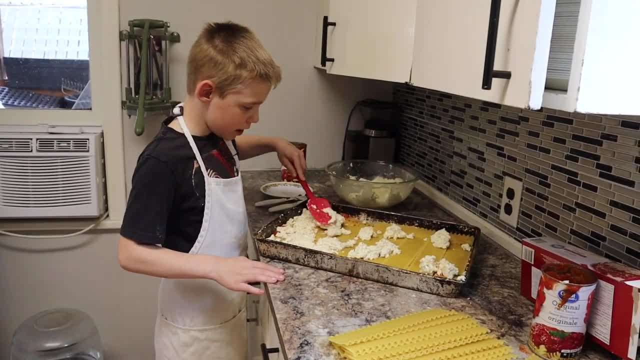 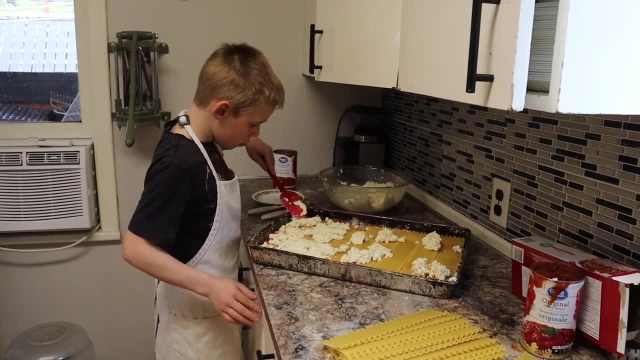 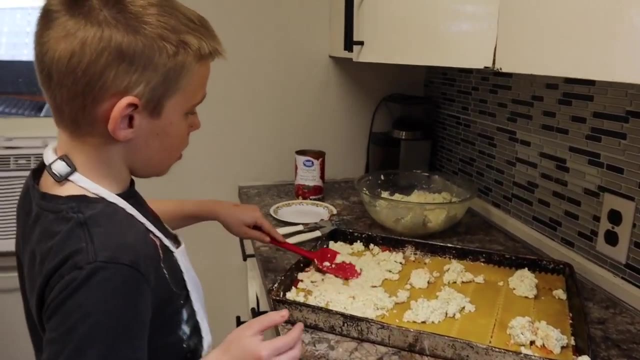 is that restaurants, you, you, you have to pay a lot, right, And there's like more- So you think the chefs make a lot of money? I think so. Would you want to be a chef, Or, or, or, or, or someone that, that, that? 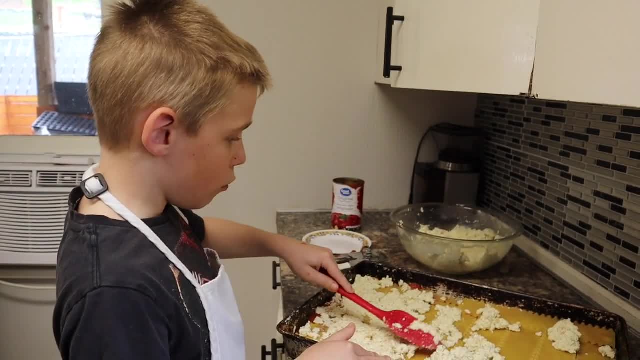 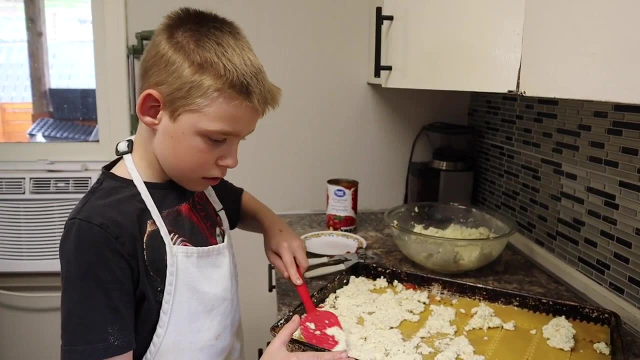 that that when someone tells order up and I'll grab it and serve it to to to the one that that acts for it. Okay, Is that a good job? What kind of job would you want as an adult? I don't know. 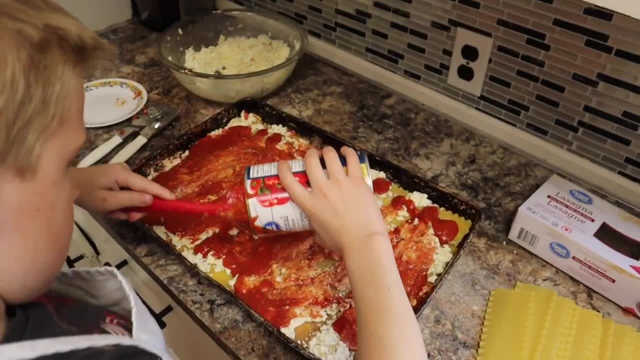 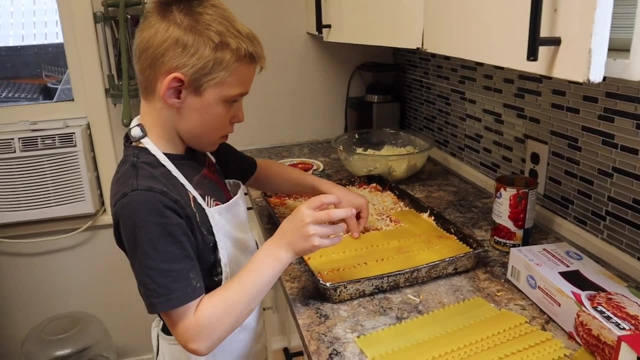 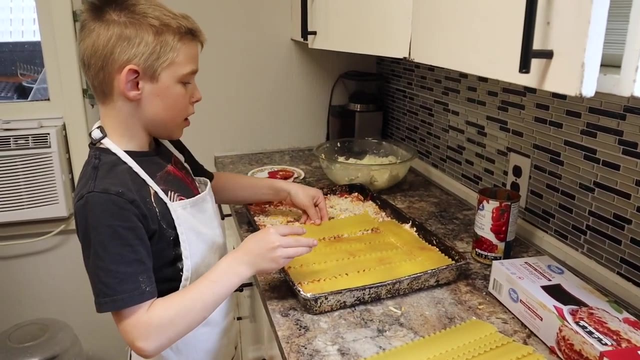 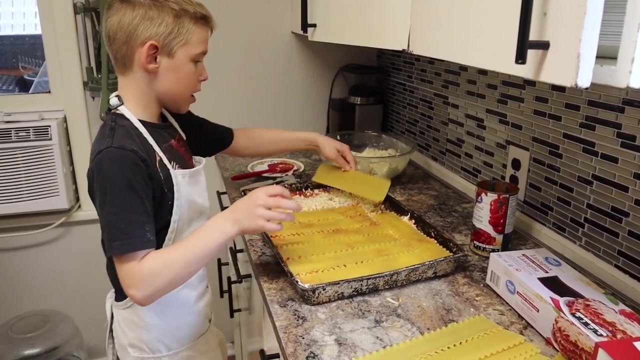 You haven't decided yet. You're just exploring your options. Yeah, So why do you think they call this recipe layers of love lasagna? Because, because it's homemade lasagna And sometimes people have heart shaped ones. I guess Heart shaped lasagna. 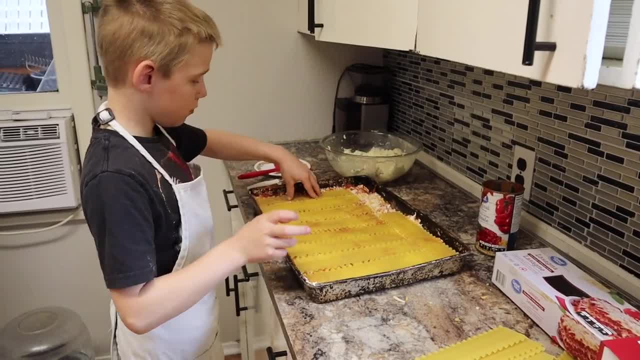 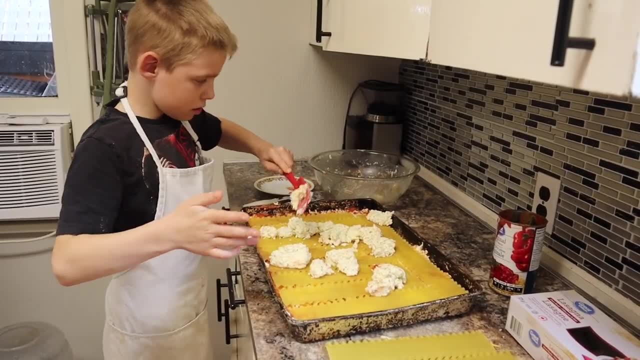 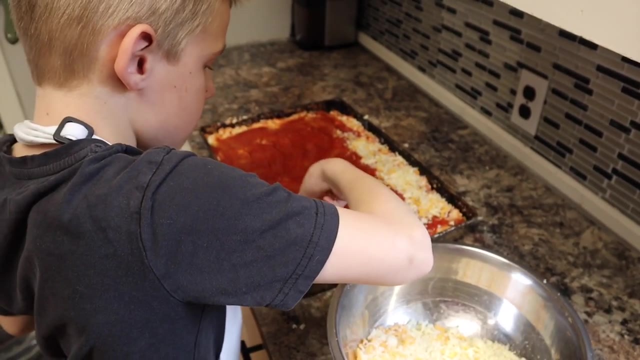 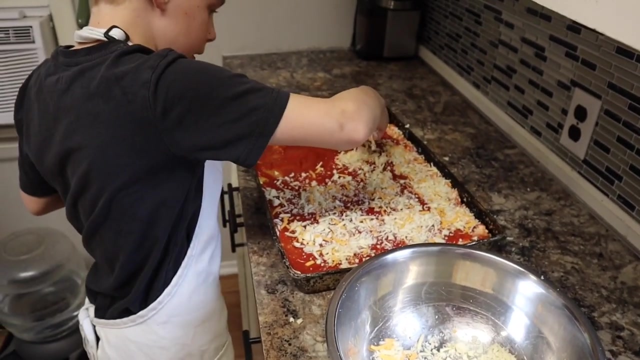 I think so. Oh, do you think because you layered everything? Yeah, That could be why. Yep, Topping it all off with cheese. Yep, Almost ready to cook this. Is it going to smell so good that it drives everybody crazy? 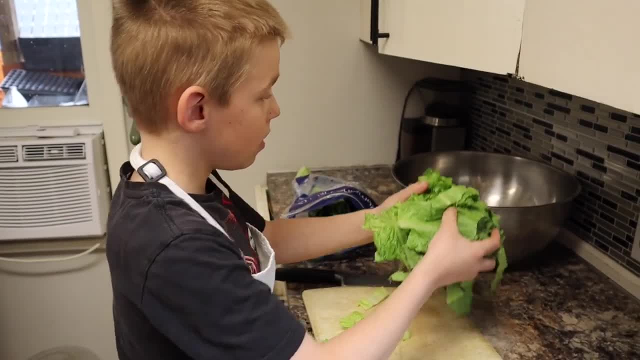 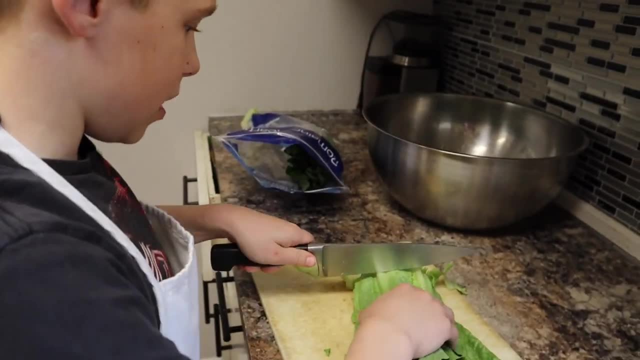 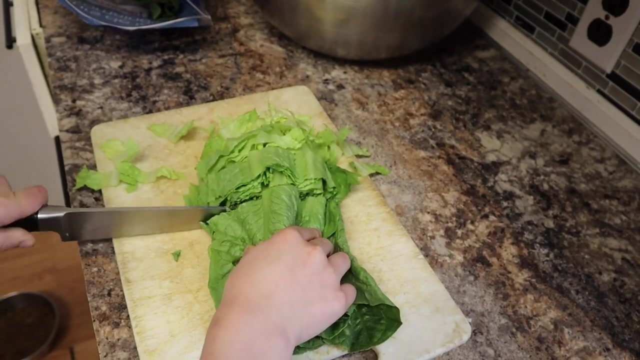 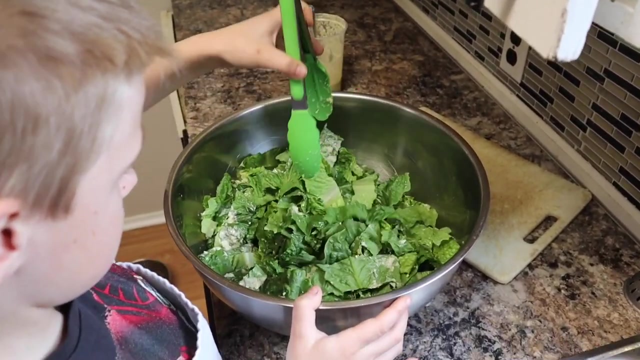 Yep, I'm making salad. What kind of salad? Caesar salad? Do you like Caesar salad? Yeah, It's okay. Please watch your fingers while you're doing this. Yep, It's a pretty big knife Getting the dressing all spread around.